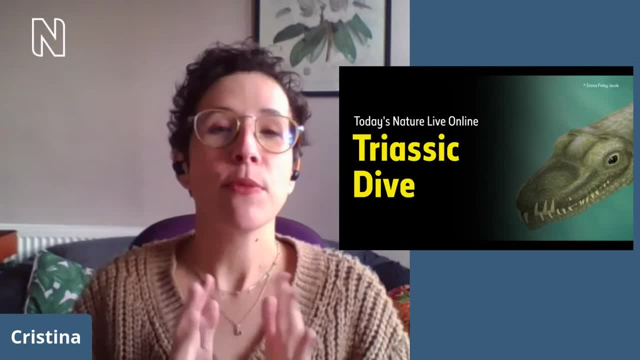 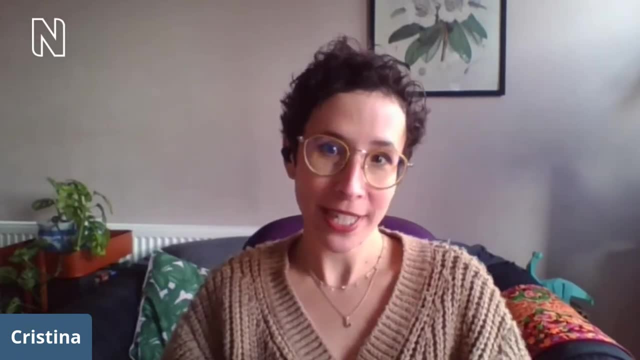 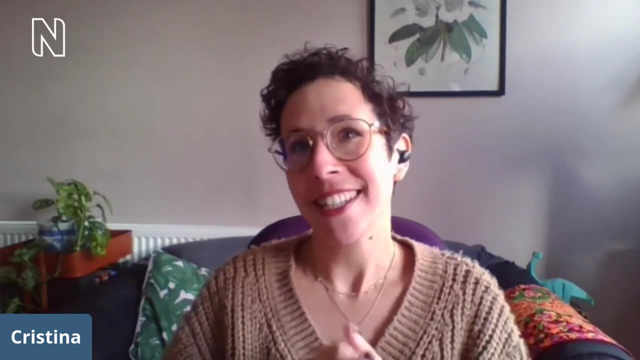 world. Today we're taking a dive in the waters of the Triassic and discovering some of the amazing reptiles that inhabit those waters, including one that puzzles scientists for years. As always as we chat, send in your comments and questions, and we'd love to hear. 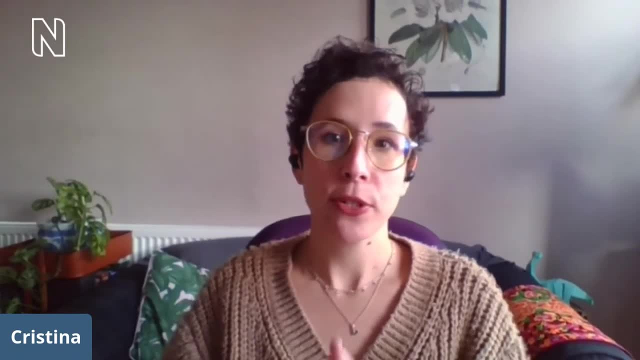 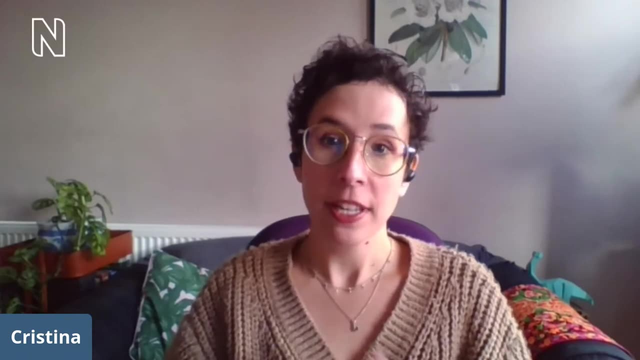 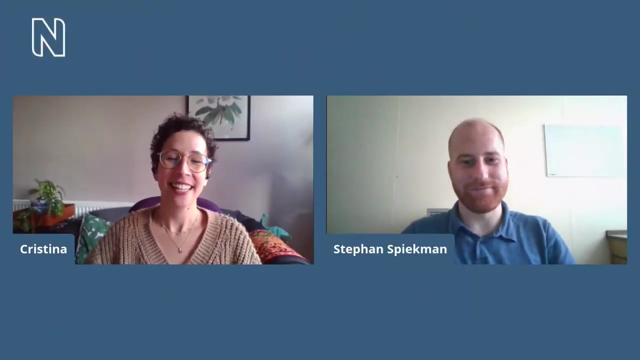 from you Now to talk about fossil marine reptiles. we have with us Stefan Spikman, who is a postdoctoral researcher at the museum studying Triassic reptile evolution. Hi, Stefan, welcome to the show. Hi, Christina, thanks for having me. 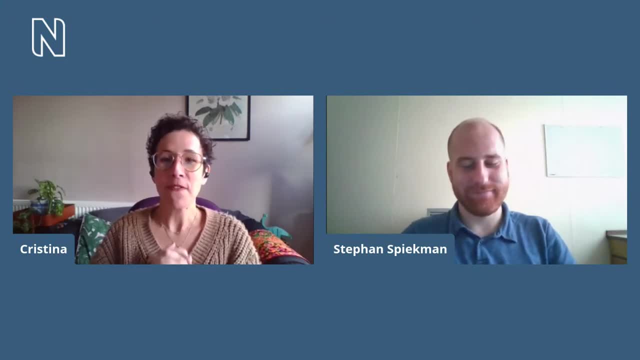 It's fantastic to have you here Now, Stefan. first things first. the animals that we are going to talk about today lived in the time of periods. they shared the earth with the time period of dinosaurs. they shared the earth with dinosaurs. they might even look like dinosaurs to their 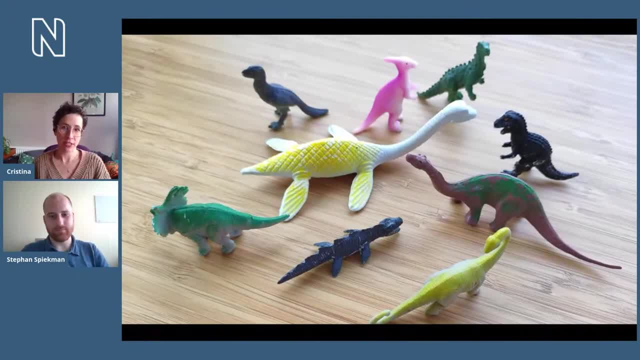 untrained eyes, but they are not dinosaurs, is that right? Yeah, that's correct. You know, we have three main groups of reptiles, right? So not all reptiles belong to the same group. So today, nowadays, we have three main groups of reptiles We have, on the one hand, we have 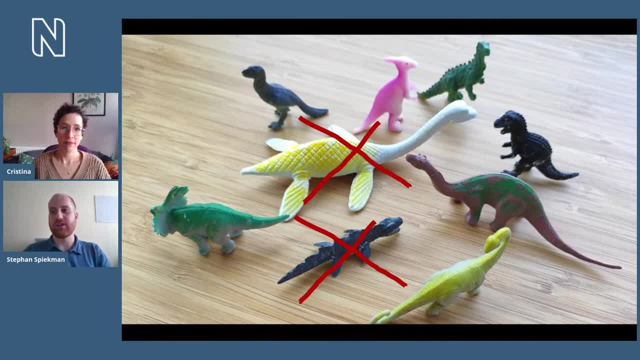 turtles. on the other hand, we have lizards and their close relatives, and then we have crocodilians and birds, which belong to another group of reptiles, to which also the dinosaurs belong. They're called the archosaurs, And similarly, also in the deep past there were 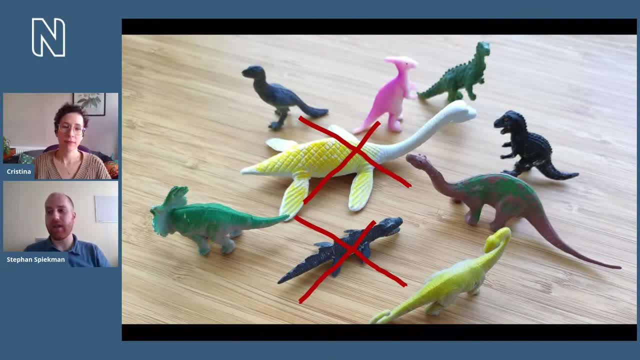 multiple groups of reptiles living at the same time. And not only did we have multiple groups of reptiles living on land, we also had different groups of reptiles going into the water, And some might look like dinosaurs because they are very big and scary with big teeth, but they're. 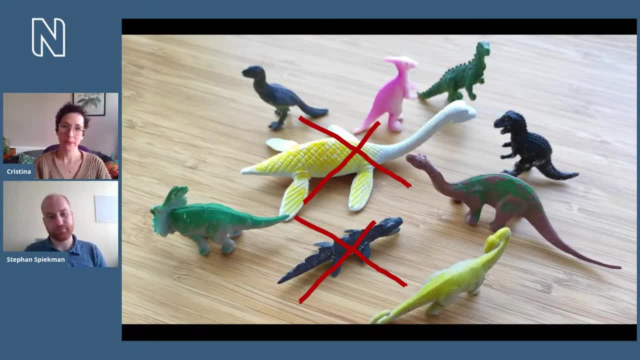 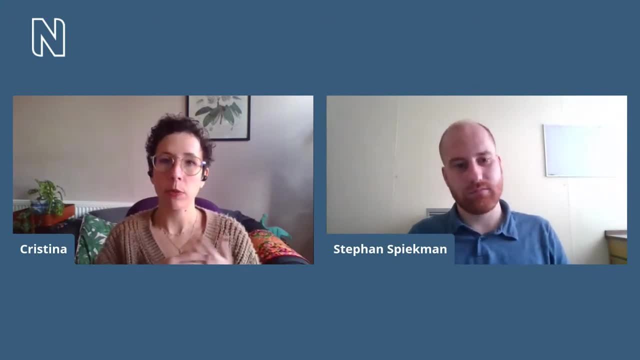 actually not related to dinosaurs. They're distinct groups of reptiles, Absolutely, And people might be familiar with some of these fossil marine reptiles, maybe with ichthyosaurs or plesiosaurs, Is that right? Can you tell us a little bit about these two fossil marine reptiles? Yeah, these. 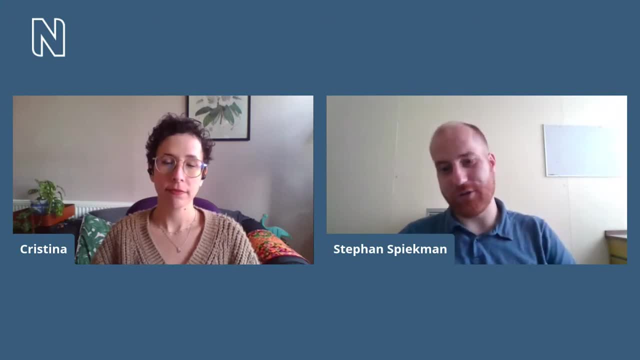 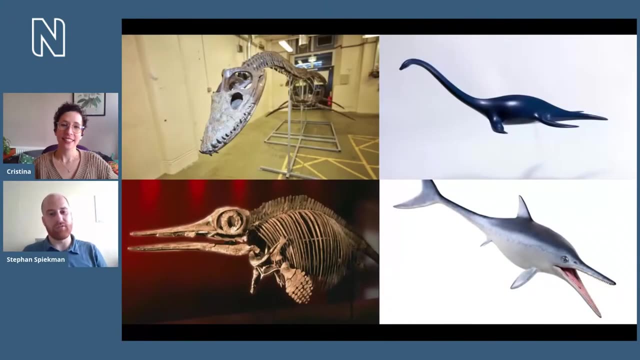 are very famous groups, especially to people who come to the Natural History Museum, because the Natural History Museum is a fantastic collection of these animals And there are two separate groups of reptiles that invaded the marine realm so that went into the waters And they're both not related. 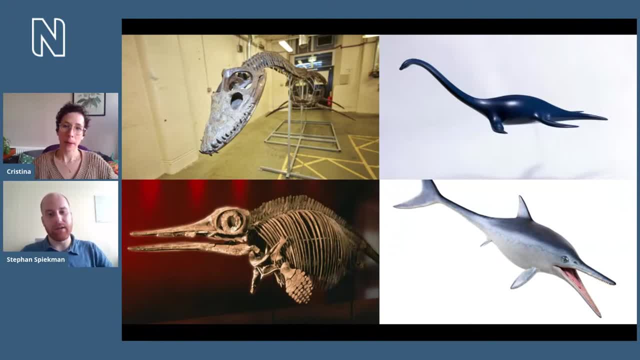 to any sort of reptiles alive today. They are independent lineages of reptiles. The plesiosaurs are quite well known, maybe even a bit better known than the ichthyosaurs, also because the animals have large necks and they look a little bit like fish, Which are actually all reptiles. 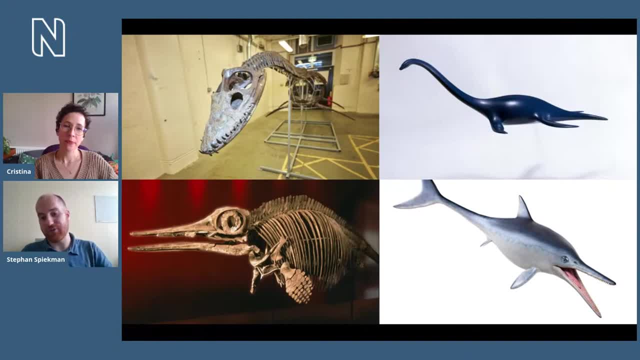 so they have Rag Мioni based on them, So they have long necks and they have flippers. And then in the bottom you have the ichthyosaurs, which kind of look like fish because they have come so well adapted to life in water that they also have a tail fin and a dorsal fin. But they're actually. 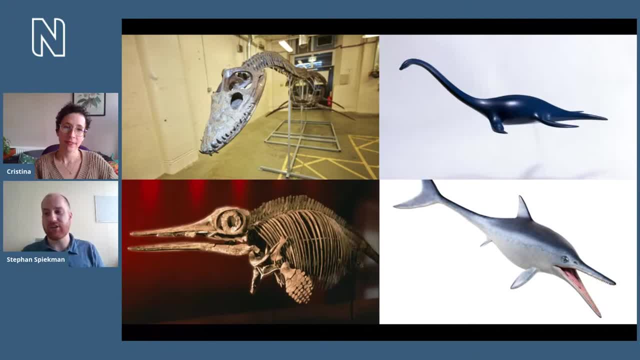 reptiles, so they're not fish at all. so you can kind of look at them as you should: Dolphins and whales nowadays, who have also similarly involved the tailfin and all of that. they look like fish but they are not fish. 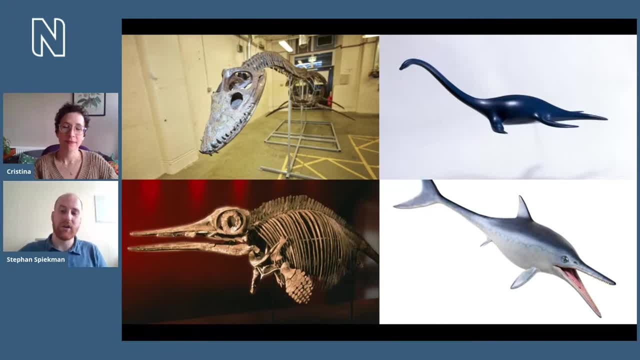 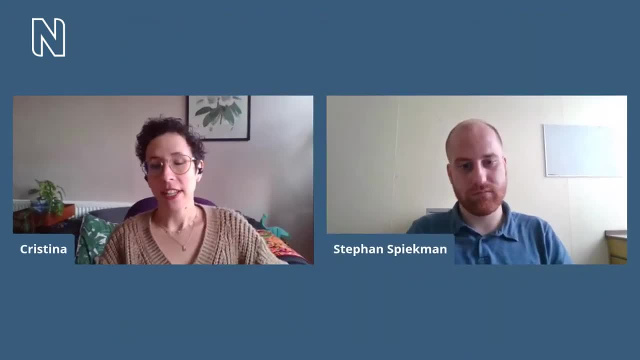 dolphins and whales. they're mammals, so they're very closely related to us, whereas these ichthyosaurs, they were very closely related to, you know, any sort of reptile, absolutely. now, um, however, um, today, stefan, we're going to be focused on the marine, the fossil marine reptiles of the triassic um. 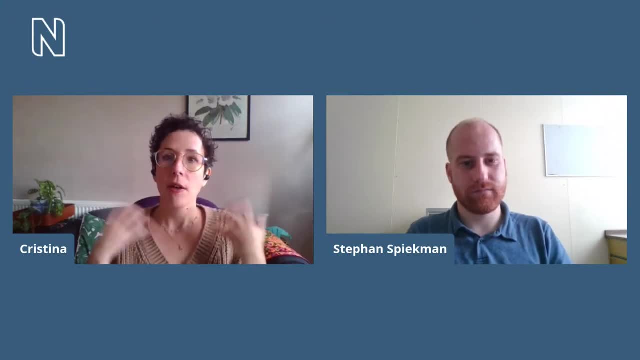 ichthyosaurs and plesiosaurs. uh, they were quite big, though there were loads of them later on in time. why is the triassic important, though? why do we want to talk about the triassic so um, the whole period of time in which the dinosaurs were also dominant, that's the triassic. 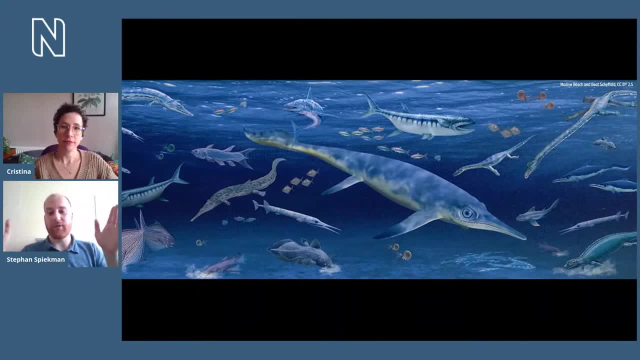 the jurassic and the cretaceous. this entire time period is called the mesozoic, and this is also known as the age of reptiles, because this was the time period when reptiles were extremely diverse and grew into these very big sizes and- and which is all- the famous reptiles. 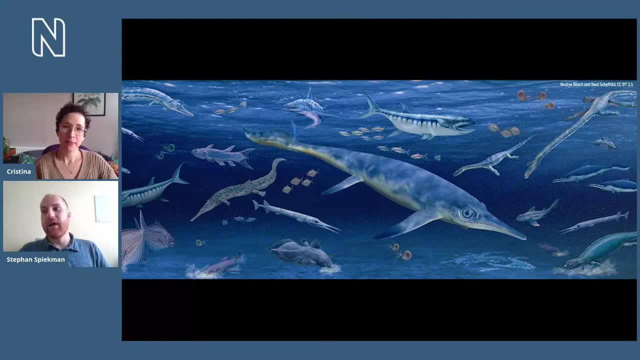 know from all your paleontology books. um and so during the jurassic and cretaceous, the dinosaurs were dominant on land and in the water it was mainly the ichthyosaurs and the plesiosaurs that were dominant. but in the triassic all of this was still developing and evolving, and the reason why 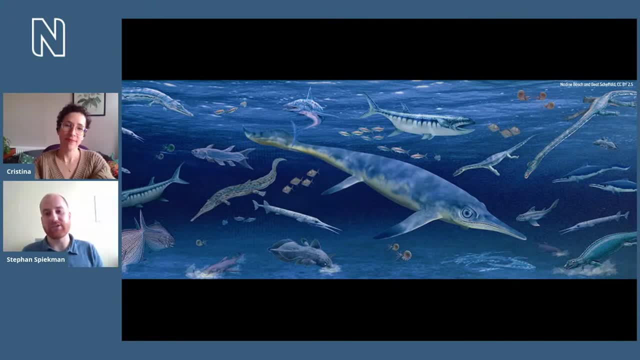 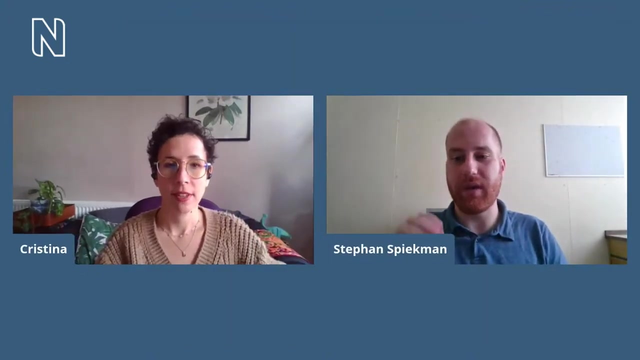 we call the mesozoic the age of reptiles. all comes down to the triassic, so many people will probably be aware of how the dinosaurs went extinct. this was due to a mass extinction event. it was most likely a mass extinction event in the history of life and the very, very biggest one in the history of. all of life was at the very beginning of the triassic. so, uh, at this beginning, at the beginning of the triassic, the largest mass extinction event that the world ever saw occurred, killing off more than 95 percent of all the organisms living in the water. and because of this, um, there was a lot. of empty space for new groups to evolve and and and occupy new evolutionary niches, right to take ecological roles. and this is exactly what these reptiles did. so, on land, different groups of reptiles evolved, which eventually led to the evolution of the dinosaurs, but also in water. 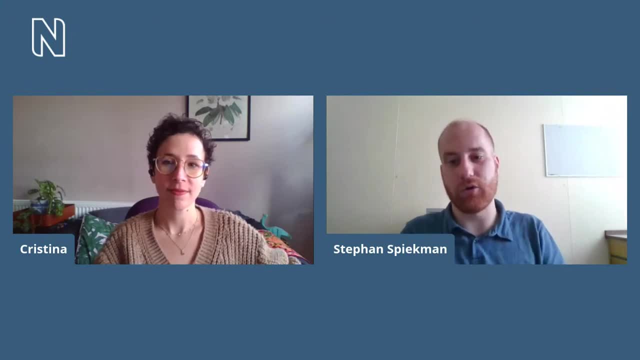 a wide array of different reptile groups invaded the oceans to take up new ecological roles, and this is what makes to me the triassic, you know, the most interesting time period, especially for someone interested in reptiles. you're not biased at all, you know um now seven you're talking about. 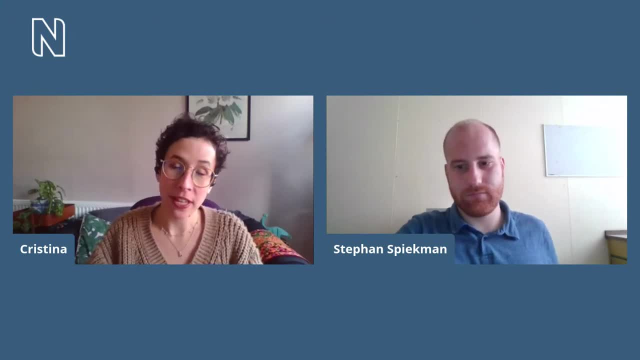 triassic. can you tell us a little bit about the, the life forms that, the reptiles, and they were alive then and how they're? they're really amazing. yeah, so we have um many, many different forms. as i said, we have some of the ancestors of the um, these disorders, and both the icky source were 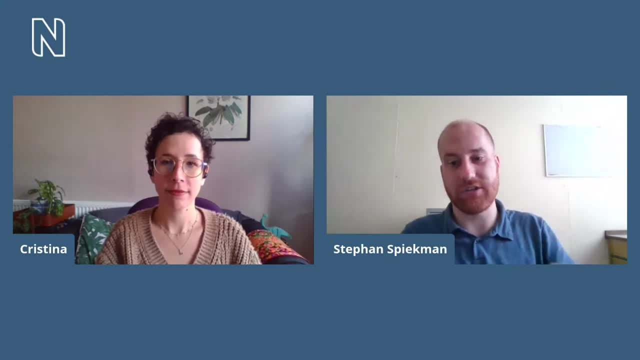 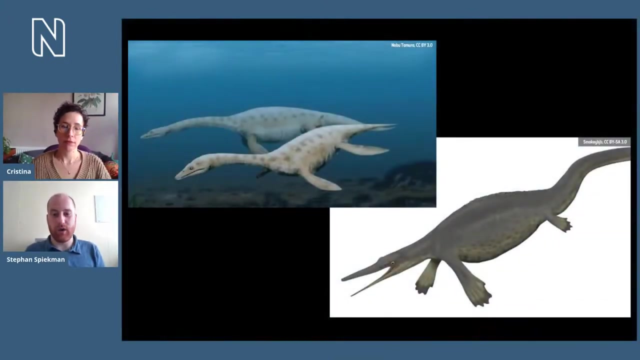 already alive at that time. so this is already the time period when their earliest ancestors were already living in the water. so we have, uh, for please your source- a group of reptiles called the piscesoroids. those are the closest relatives of um of the plesiosaurus, and when it comes to 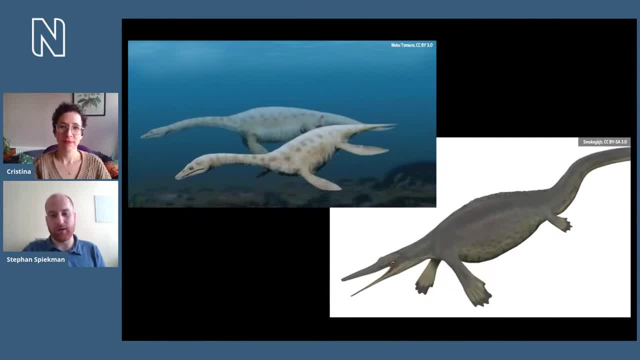 the ichthyosaurs. as you can see, in the bottom right we have these very weird looking animals called hupusukians. so you can see that they are maybe a little less well adapted to life in water than the later ichthyosaurs are, but they are very closely related to them and those hupusukians is 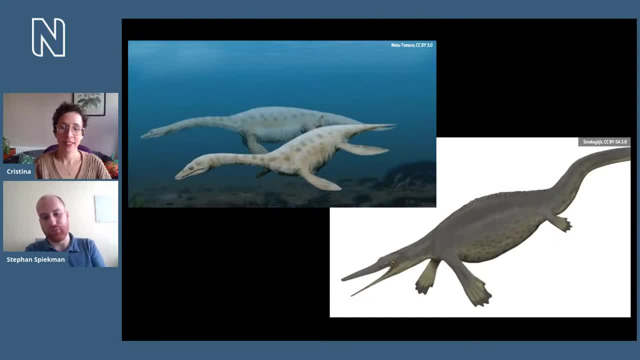 really a group we've only been finding out about relatively recently from new fossils from china. that's amazing. you can see the the similarities, even for the untrained eyes, for those of us who are not um a paleontologist, uh, but yeah, it can be there. and now there's another group that i, i really wanted you to talk about the placodons. can you tell us a little bit about these bizarre reptiles? yeah, so, arguably the the most diverse group of marine reptiles during the triassic was the group of reptiles to which the plesiosaurus also belong. so this bigger group in which the plesiosaurus fit, 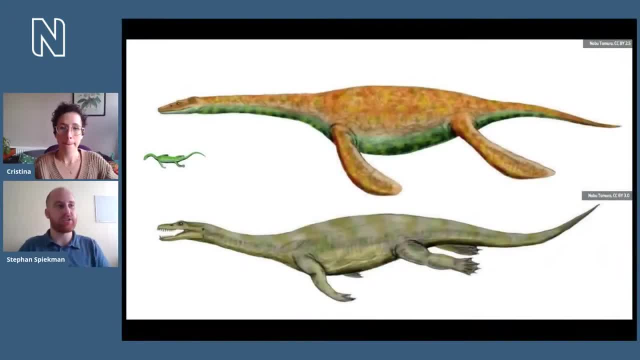 is known as the andocteridia. so these included, these pistosaurs that we just looked at, but also, uh well, the animals we see here, which is again a pisces or a pisces, or at the top and then the bottom, we have anothasaur, which was quite a common animal at the time and was a predator. 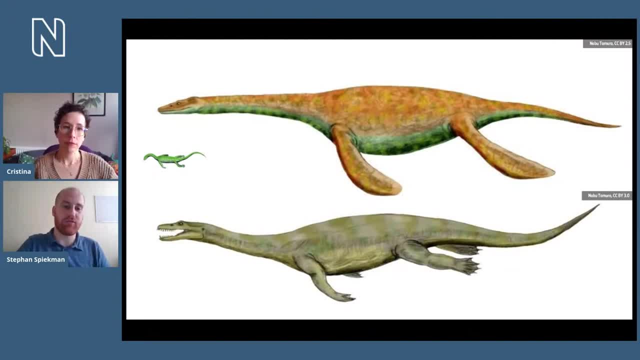 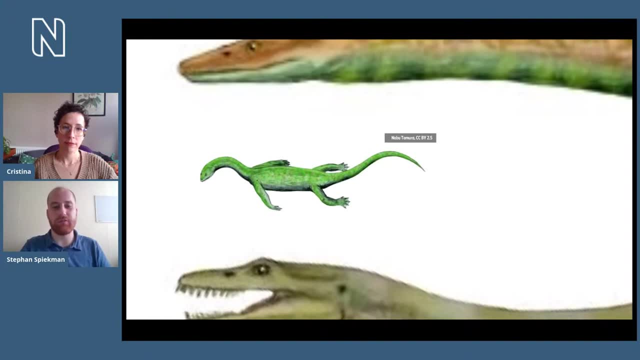 eating fish and prey, like that. but we also had very, very small forms like the pachyplurosaurus that you see here zoomed in now. so they came in all different shapes and sizes and we have many, many fossils of these animals. for instance, from the time of the early 20th century there was a very small 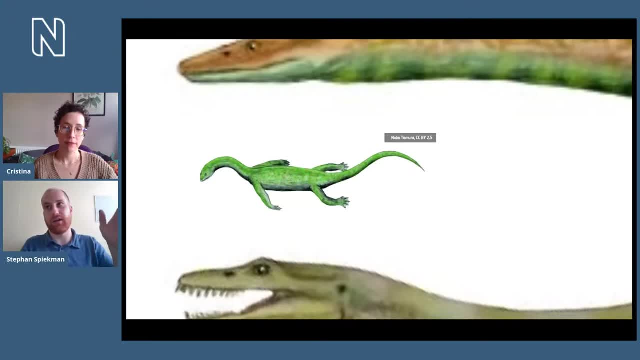 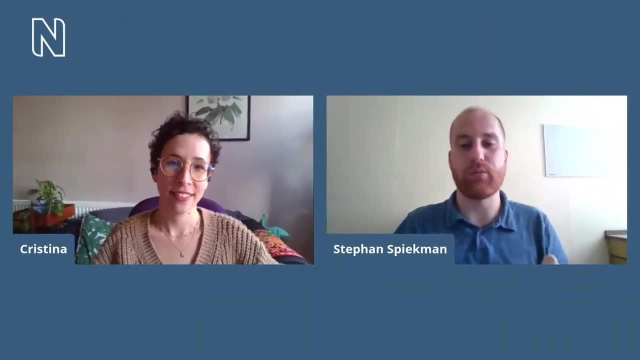 small guys, the packet blurs, or we have an entire uh um ontogenetic series, so entire growth range. so we have them from small embryos, actual fossilized embryos, all the way to the adult animals, but then the animals you mentioned, specifically the placodons. they're also very 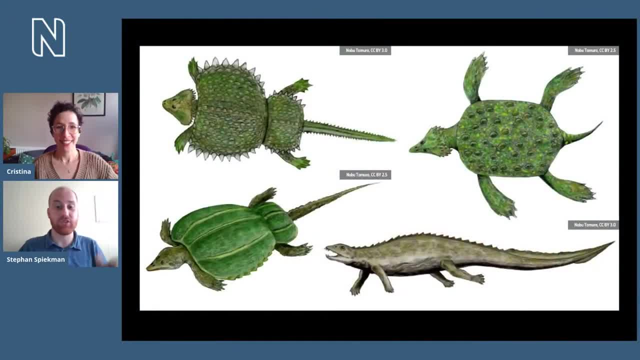 interesting. they're a different form of um subterranean and, as you can see, they're very weird. they were armored, so they they kind of resemble turtles in the sense that they have a carapace, so they have like a full-on shield of armor, um, but they're actually not turtles as. 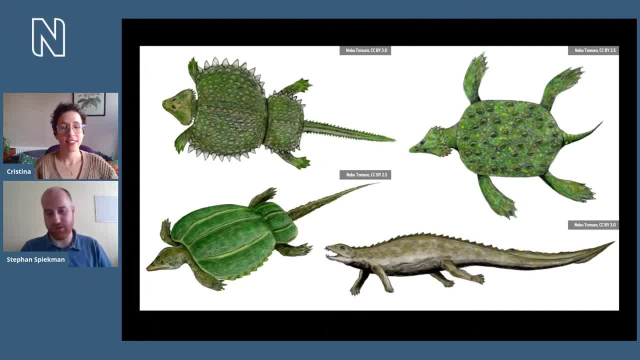 i said, they're served origins, so they're close relatives of the plesiosaurus and these other reptiles we just looked at, and they independently evolved this type of armor that completely covered their bodies. another interesting aspect about these animals is that they had very large 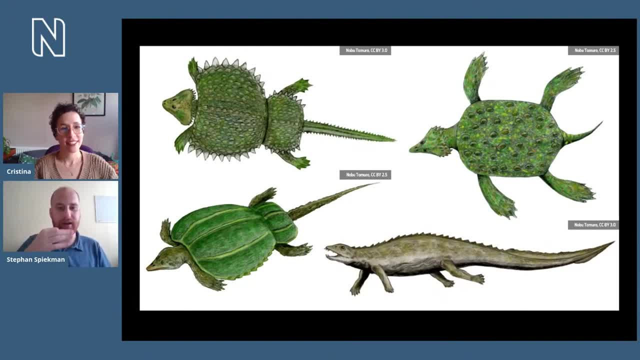 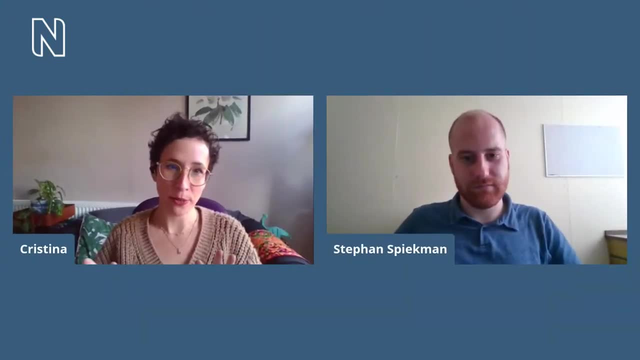 crushing teeth that almost looked like just rocks in their in their mouth that they used to crush, uh, the things they ate, which was mollusks and other shells, uh, so really bizarre animals that were around at the time. that's amazing. and the seven, just to triple check, these are not related to turtles then that much, apart from them being reptiles. no, no, so. 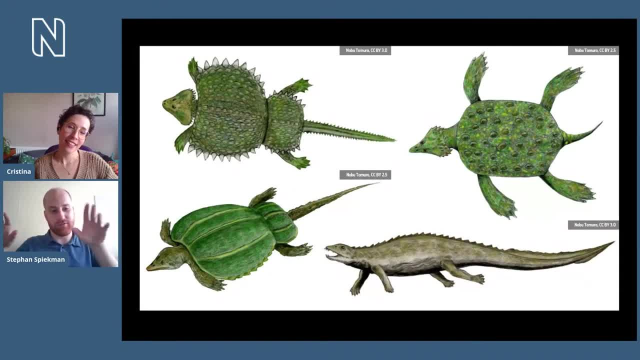 kind of in a similar way that both ichthyosaurs and dolphins evolved this fish-like shape. in the same way, both the placodons and the turtles evolved the shell separately from each other, and you can also, when you look at fossils in detail, you can see that they evolved in a different. 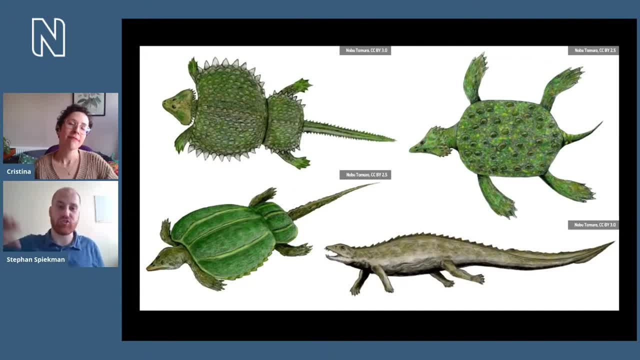 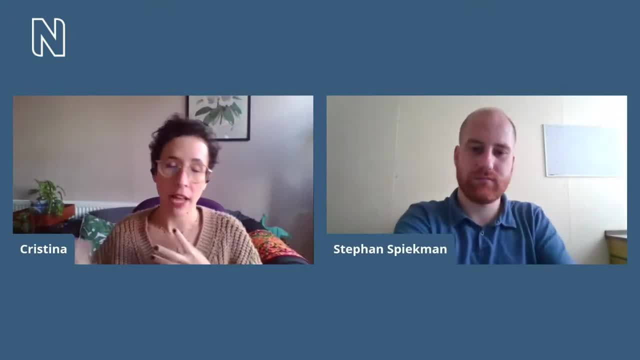 different way. so so turtle shell, slightly differently constructed than these shells are, and, uh, these wide diversity. we've seen big animals. there's more animals, animals that resemble all the animals. some of them didn't make it to after the triassic, did they? um, this is an example that i think it looks beautiful, at least. 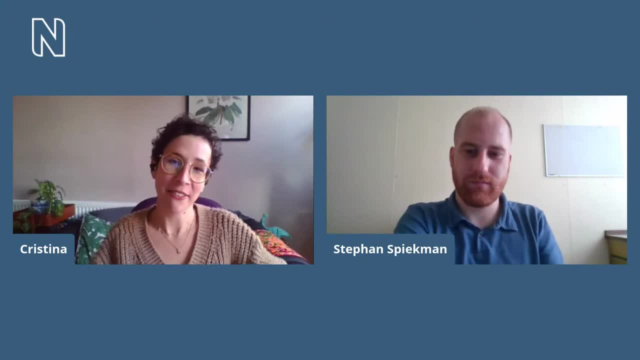 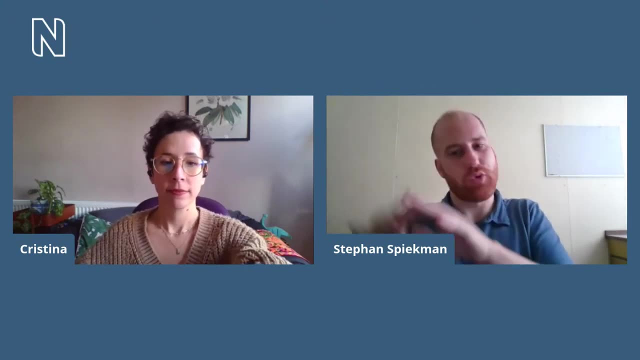 the representation that we had for sally. it just stayed in the triassic, is that right? yeah, so the in the jurassic and the cretaceous. we were basically left with the plesiosaurs and ichthyosaurs and some other groups, but many of those groups that evolved in the triassic never made it into the jurassic. they 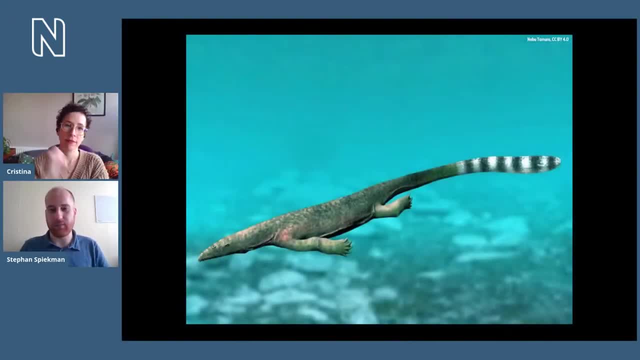 they evolved early on and and then went extinct by the by the time the triassic came to an end, and one of the animals we're looking at now is called the philatosaur. they're also marine reptiles, which is a bit confusing, which are called philatosuchians. those are crocodile relatives, but 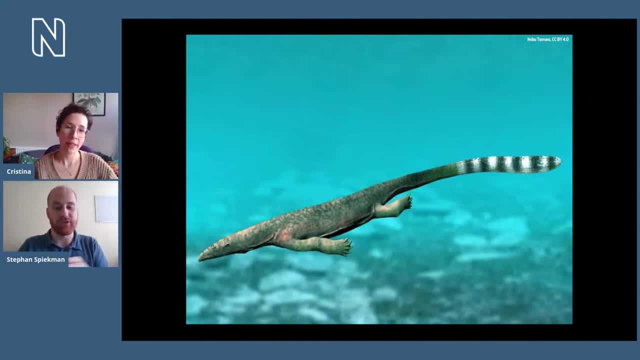 those are not the ones we're talking about. these guys are called philatosaurs, and philatosaurs kind of resemble crops a little bit, as you can see, but they're not so they're not a completely different species of reptiles that in the triassic, went into the marine realm and evolved to live there. 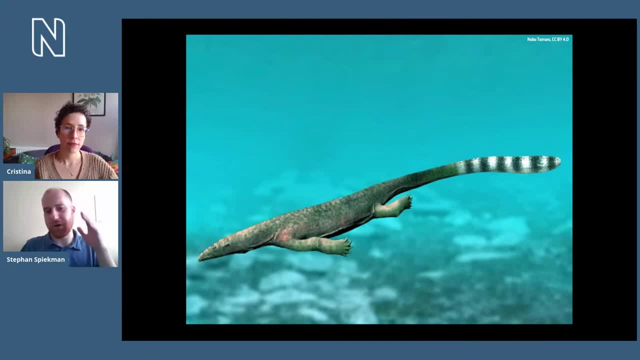 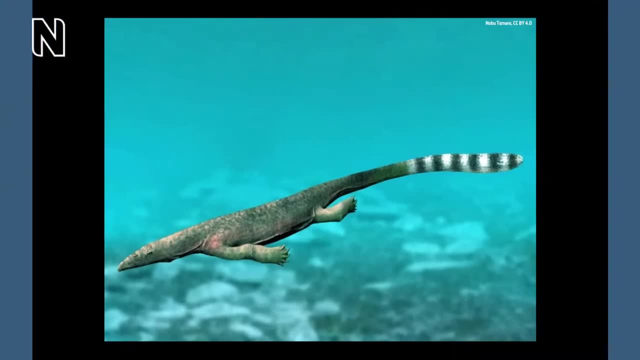 and the interesting thing about philatosaurs is that they have very weird skulls. so we have different species that have different shaped snouts, different shaped skulls and different teeth, which indicated they were actually quite diverse and eating on a wide range of things, so some might be more suited in crushing shell prey, somewhat like a placodont, less extreme, but more or less. 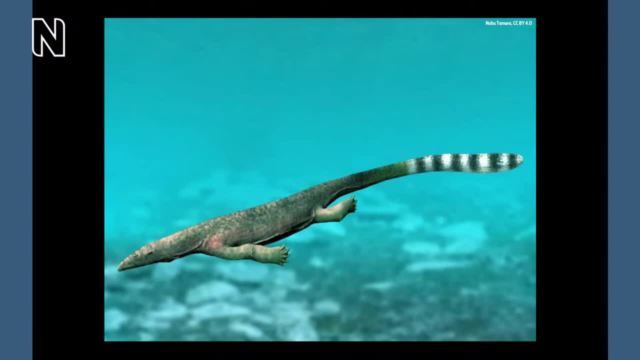 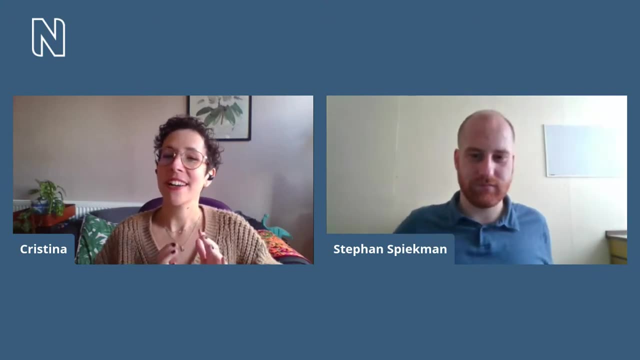 the same, or others were maybe more evolved to feed on fish, and and so on and so forth. so for them we're talking about philatosaurs, and philatosaurs have a very unique shape of human body. they have a very SMALL, tiny head and they have a very large mouse, and so on, and so 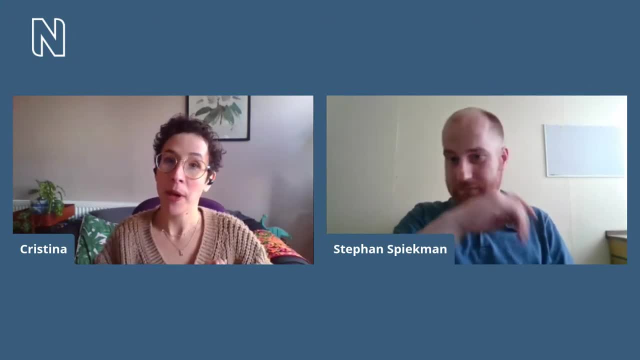 forth, and there's a really interesting part about the philatosaur species that they have and when they live they they live in these deep bottom lobes and so on and so forth. so I think there's a lot of different things about them, um, and obviously, I think one of the things that we're 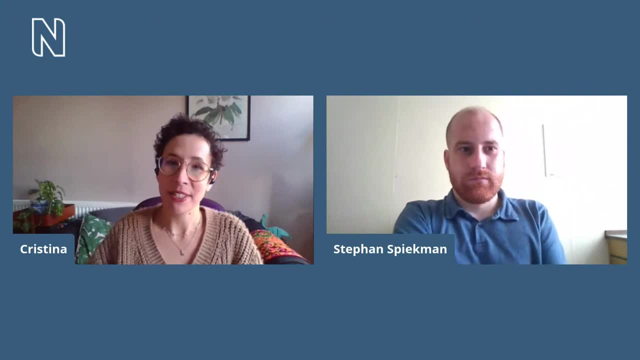 looking for is an egg, and I'm curious to know if one of the species is an egg and is that a different species? or is it a different species or is it not different species? to the museum? you can do so by clicking the button uh near the chat on youtube or going directly to. 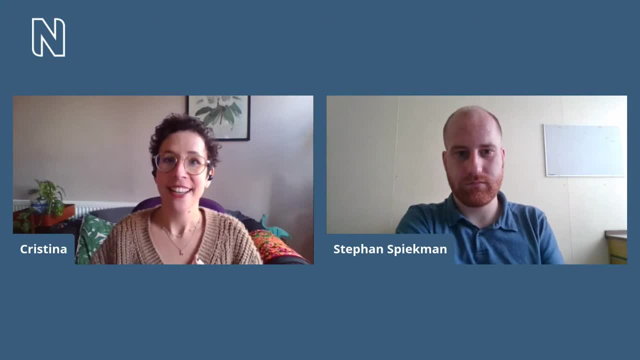 our website and we'll put uh an address on the chat so you can click in there, and any donation is always appreciated and if you're enjoying the show, what a better way to say thank you? but, um, stefan, going to the questions, um, that obvious. we're sending um my next set. we're asking how. 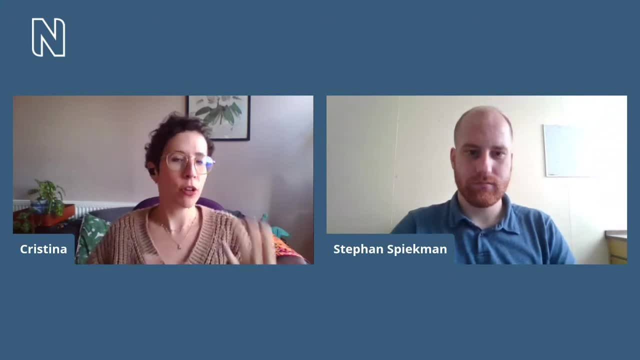 can you tell that they are reptiles? so we were talking about how we know they're not mammals or they're not fish, but what makes them, um, reptiles? is there a particular thing that you can go? yep, this is a reptile and this is not a reptile? um, that's a very good question, and it's actually. 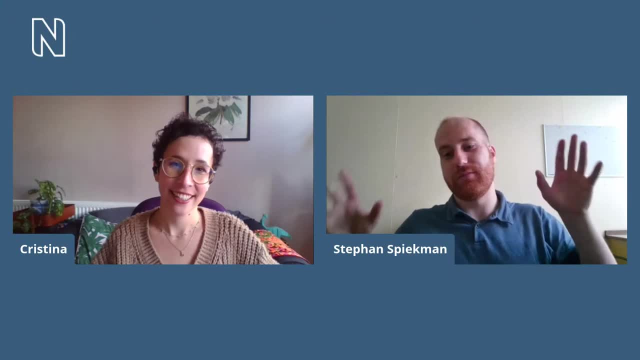 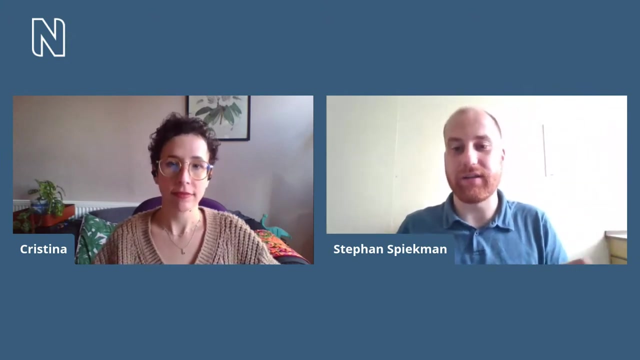 very fundamental, obviously. so everything we do as paleontologists is what we essentially do is we try to group all the animals, both living and extinct, into the right evolutionary uh categories. uh, in terms of reptiles, there are a number of uh character traits um that we find that are: by most reptiles. but the deeper you go in time, the more murky this gets. so, for instance, all reptiles nowadays- and now nowadays- are all what we call cold-blooded, so they have a very slow metabolism. but as we go further down in history and we look at the bones in more detail, we do more. 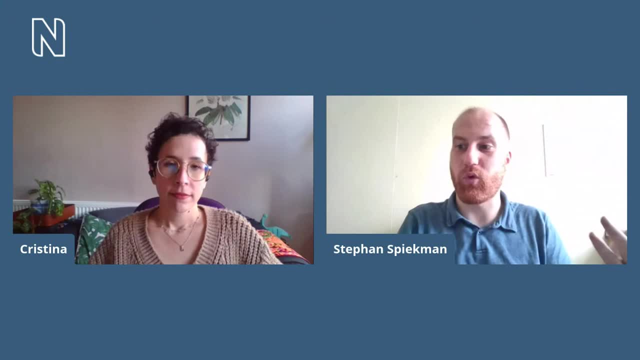 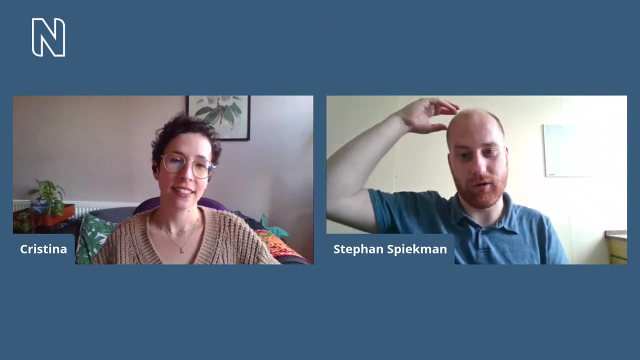 analysis on them, we actually discovered that there were even reptiles, were somewhat warm-blooded, so this is not a very easy question to answer. one um one answer that that works as a rule of thumb, for is that, um, there are, in the back of the head, there are openings that were openings that are 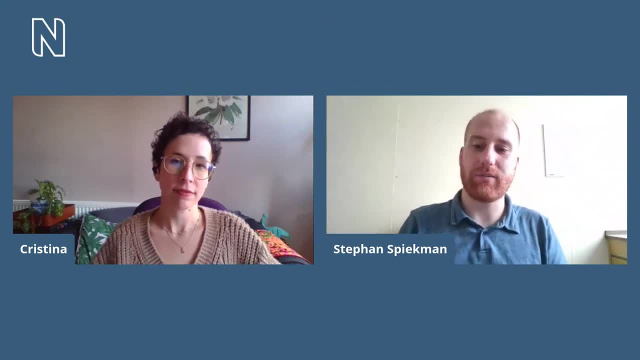 basically spaces for muscles to attach, and almost all reptiles have two openings. so we humans and other mammals, we have one, which is your, your temple. you can, you can feel that even so, when you, when you close your mouth, you can feel the muscles moving there. that's because there's 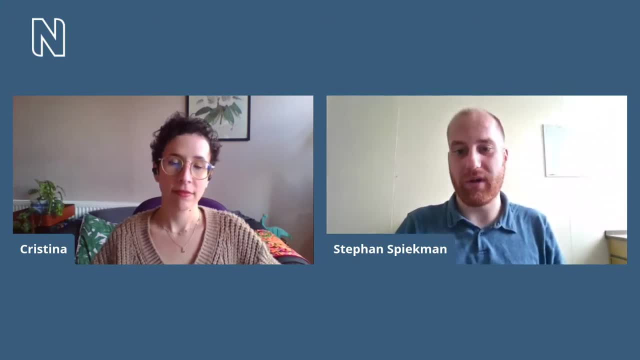 an opening in the skull there. so most reptiles have two openings um, which is one of the main character traits we use. but again, there are exceptions to the rule, because biology, yeah, likes to not stick to rules. as always, biology likes making it difficult for for the 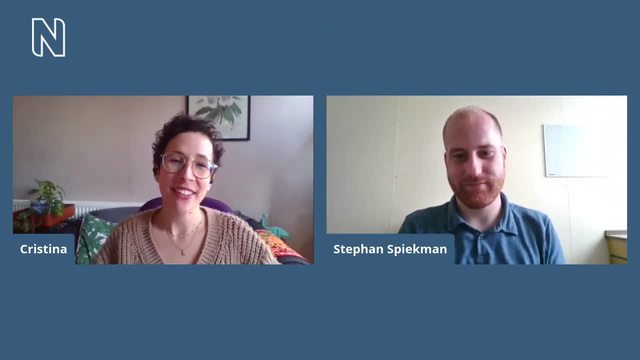 researchers, i think. but that was that. that was a great answer. uh, stefan. another question, this one from andrew. they were asking what would have had a more powerful bite: a big sea reptile or a t-rex? can we tell even gosh? um, yes, we can tell, there are ways of reconstructing uh bite, bite force in. 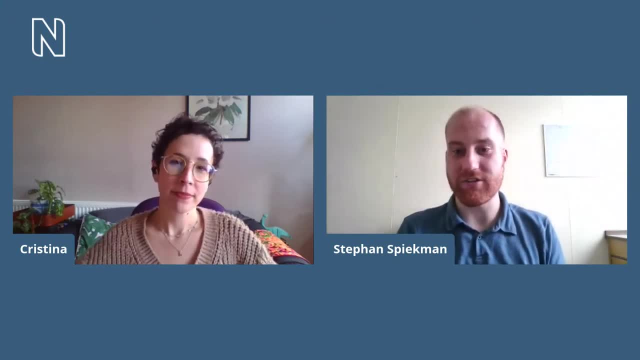 in in reptiles and extinct animals generally, and there's a lot of very good looking species, of species of sea reptiles and um, but i'm not sure, um, if it's been done for, please, the source. i don't have this uh knowledge off the top of my head, but 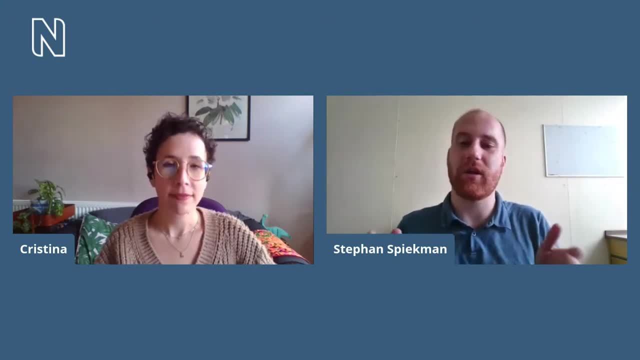 my expectation is, um, that pleaser source would not have as strong of a bite. i mean, it depends on the type of pleasure you're looking at. uh, please, most pleasing source. they have a quite a small head at the end of a long neck and what they ate was things like fish and squid. so what? 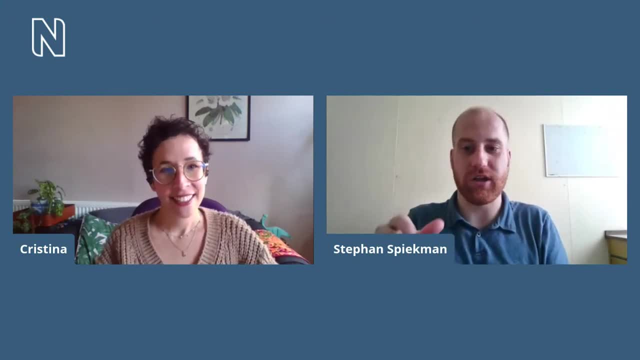 they needed. you can also see this in their teeth. they have these very long pointy teeth which are like fishing spears, so you close your mouth, fish gets caught and can't go anywhere, so you don't need a lot of bite force for that. a t-rex, on the other hand- um you know, was also crushing bone and and hunting big, uh, other big dinosaurs, uh. so in that regard, uh, t-rex had a very strong bite, but there were also some marine reptiles out there- maybe not the long-necked plesiosaurs- that had very strong bites because they were also hunting very big prey. that's brilliant. that's a. that's a. 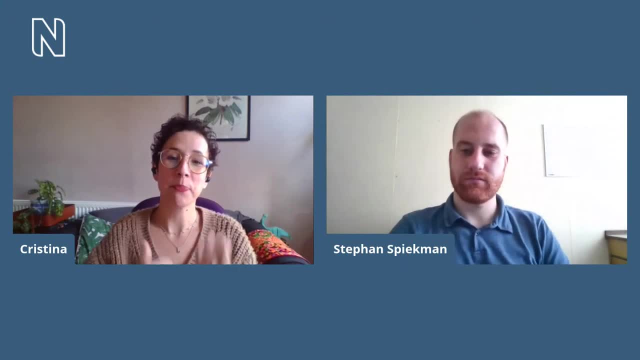 great answer as well. so, yeah, if anyone has any more questions, please send them through and we'll. uh, we'll try and answer them and, in fact, um stefan. just now another question arrived. this one is from bethany. uh, they're asking: are the colors using the artistic images based on? 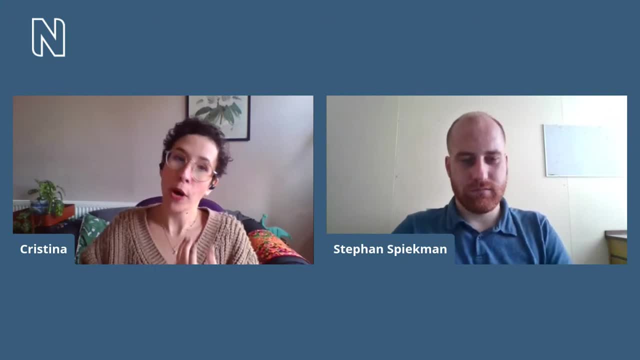 scientific research or artist rendition, or both do. do you know if, like, the colors are approximate or, yes, would change in the future? yeah, so um, until very recently, we were always saying, as paleontologists, you know, we will never be able to say anything about the colors that animals had. uh, simply because the color itself doesn't preserve. and also, 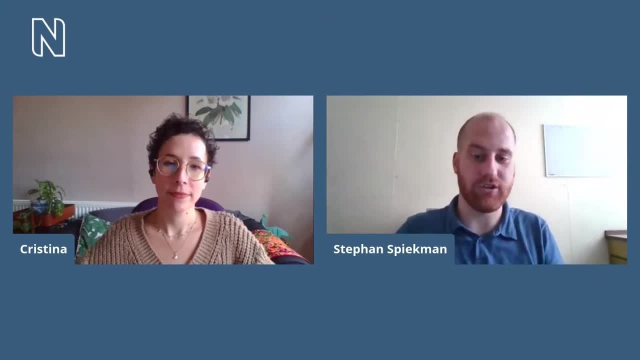 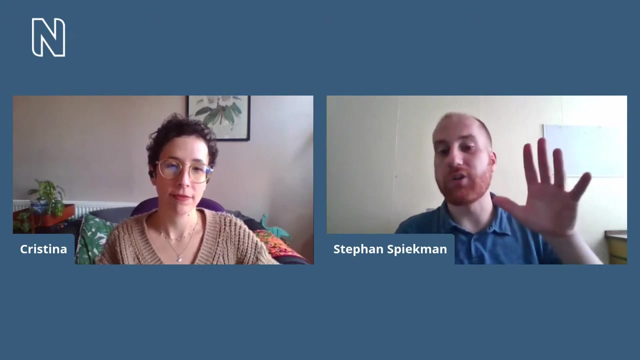 things like dna that you can use to to figure out what color something might have had are not preserved in in fossils that are this old. however, there have been really exciting developments in the in the last like 10, 15 years, where there are certain um biological structures. 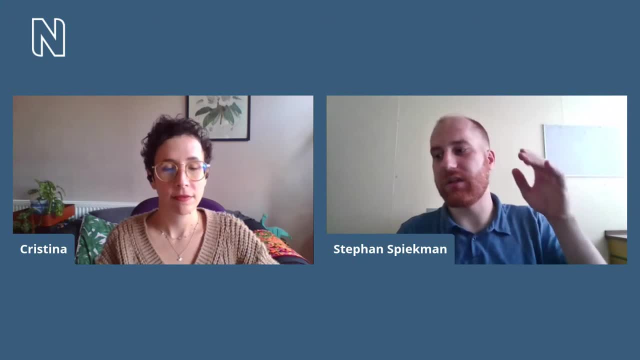 uh, uh, maybe remnants of certain proteins, even that that um or uh of of things that indicate color that we have discovered in certain uh fossils. so, for instance, for certain dinosaurs, we've now been able to give a rough estimation of what color they are. for marine reptiles, this 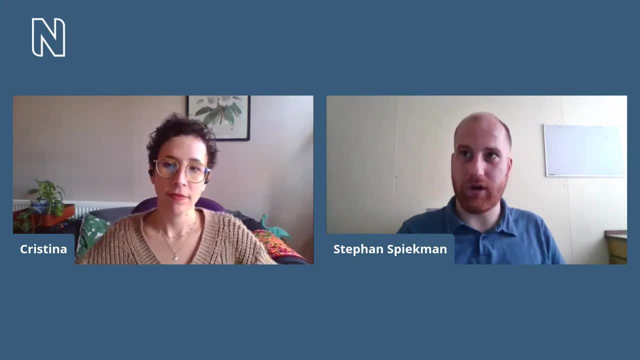 so far have been done on, or we have not been able to do this in this level of detail. however, there's one example i know of an ichthyosaur where um- i think these were melanosomes that they found where they could indicate they could see that um on this ichthyosaur, the top half of the 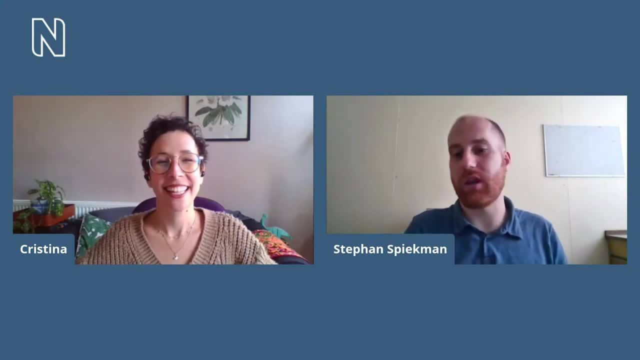 body was a darker color, whereas the bottom half the body was a lighter color, and this is not surprising at all. this is also what we see, for instance, in in many sharks and fish today, like if you look at a great white shark. it's white from the bottom and dark from the top. and why? 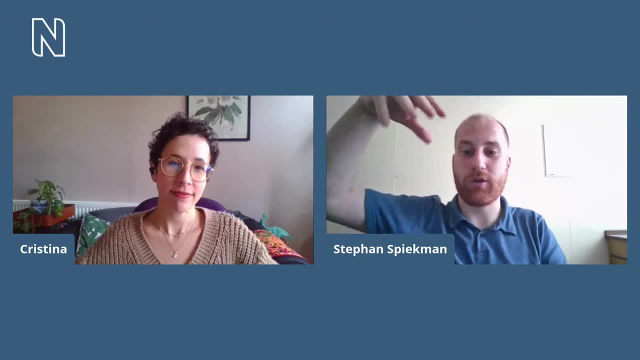 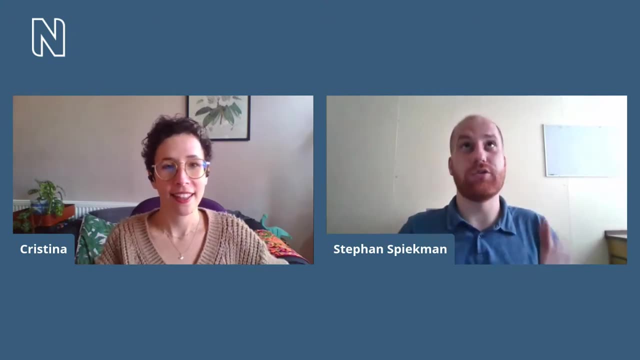 is that? well, that's because if you look- uh, if you're in the water and you look down, then you see the darkness, whereas when you look from the bottom and you look up, you see you look against the sunlight reflecting on the water, so there's a much more of a light. 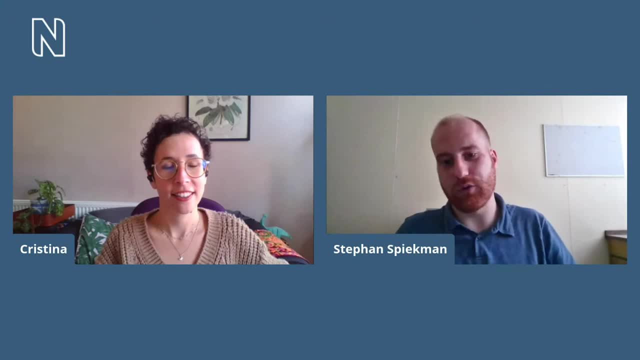 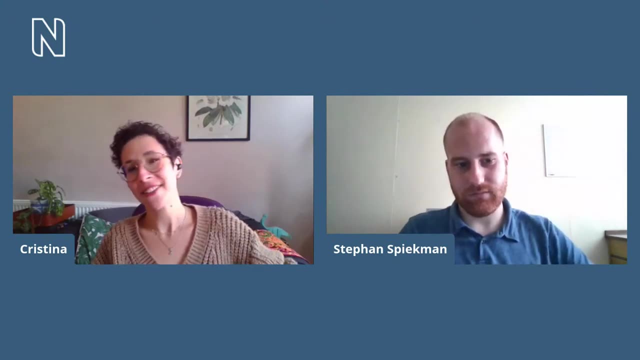 background. so you see that these animals, uh, you know, to a certain extent, uh, we're doing the same thing that animals are doing nowadays. fantastic, that's. that's an incredible answer and it's something, it's a question that i've heard a lot of people asking in the past. so, yeah, thank you. so. 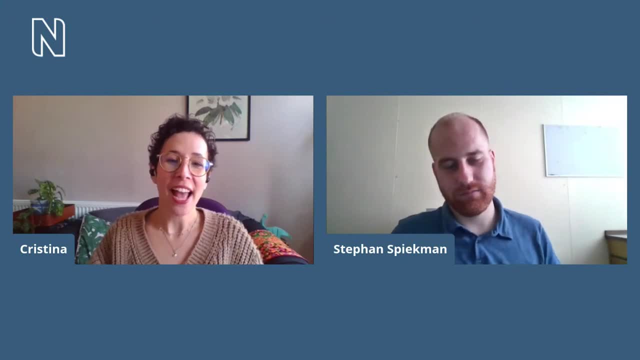 much, uh, stephen. one last question before we continue. and noah, who is seven, uh, is asking when megalodons around before. do you know? but you're not a megalodon expert, but do you happen to know the time when megalodons? 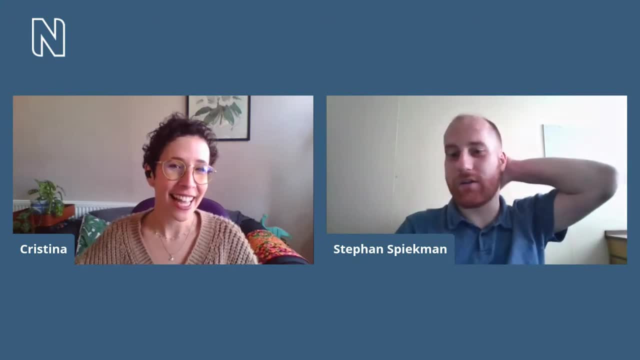 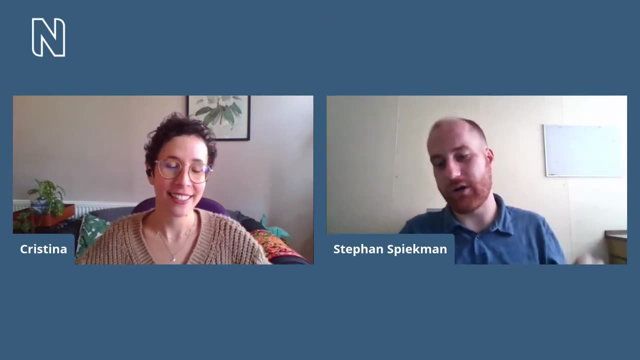 were around. i can't, yeah. from the top of my head, megalodon was actually a very, very recent animal. there were already ancestors of direct ancestors of us, of humans, walking around on the earth when, when the last megalodon were still swimming in the ocean. so for those who don't know megalodon, 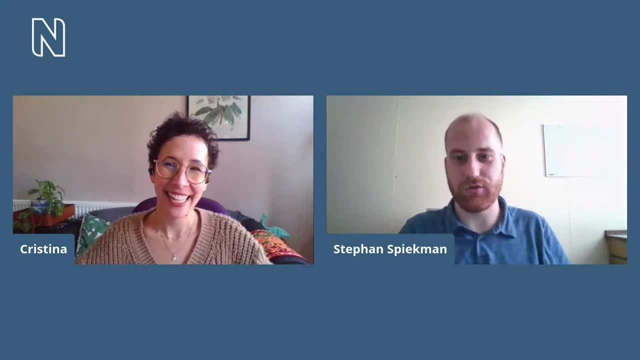 is an enormous, uh, predatory shark, close relative of a white shark, but it was extremely large and it you know things like whales. it was a very impressive animal. so sharks as a group are very, very ancient, much older than any sort of reptile, so there were definitely sharks around. there were 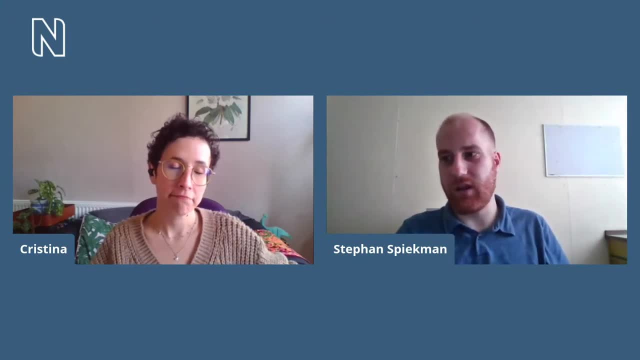 also big sharks around, uh as well. nothing as big as megalodon and also nothing really closely related to megalodon. so the types of sharks that were swimming around back in those days were looked quite different than than megalodon or a great white shark does. brilliant. thank you so much. 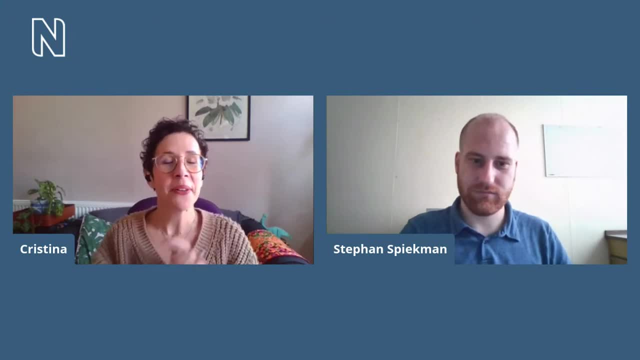 stefan, and thank you everyone for for your excellent questions. now, uh to uh go back to what we were talking about. we're talking about the triassic reptiles and marine reptiles, and there's one in particular that again not by us at all, stefan, but we wanted. 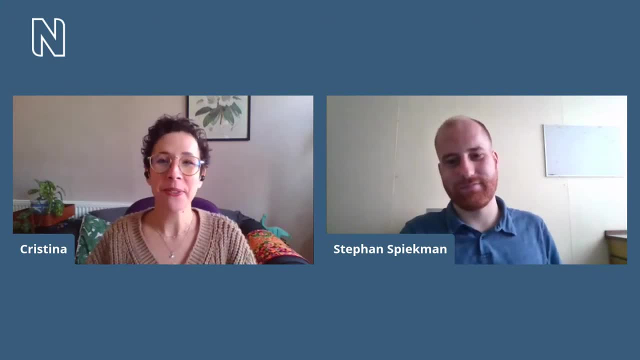 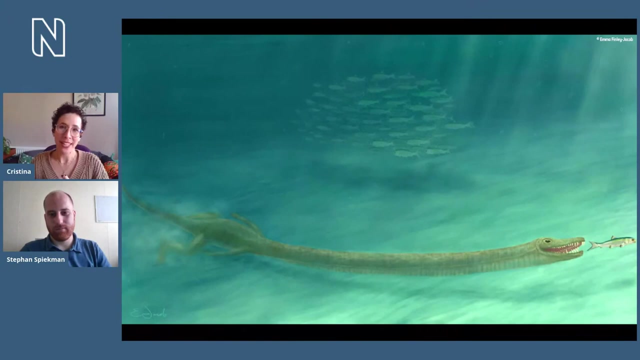 to talk about? uh, because it's, it's. it's a really cool marine reptile and also it got scientists puzzled for a long time because it's a little bit bizarre. and this is tanistrophius. it's a reptile that you've been studying in particular, so can you tell us a little bit about tanistrophius and what? 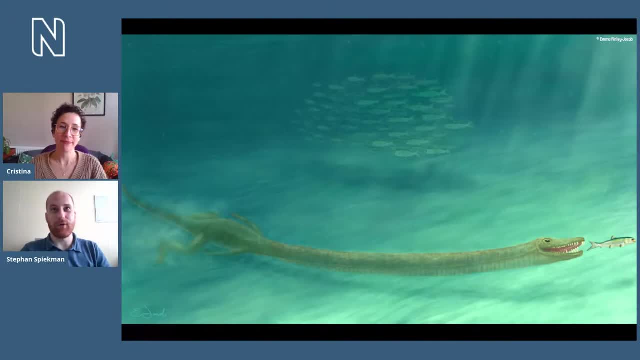 they're sure, stefan. yeah, so tenestrophius is the animal. uh, i studied like a large part of my doctoral degree, so my phd research focused on this animal and, as you can instantly see, tennis trophies characterized by an extremely long neck, like those pleases, are, however, the 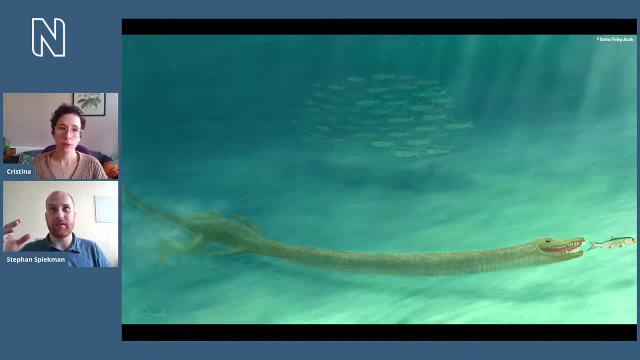 thing with tennis trophies is, it was, um, it evolved this long neck in a very, very different way, which we can see in a little bit when we will look at the skeleton. but it has a very, very long neck and, uh, in contrast to things like pleasesource, it didn't have paddles, it just still had hands and feet. 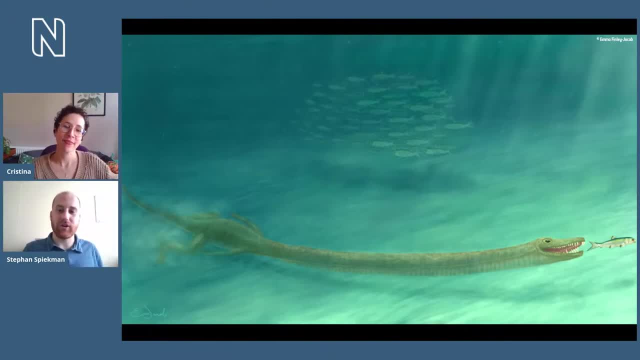 like reptiles living on land do, and um, we actually also know how it's related to other reptiles. tenestrophius was actually very closely related to modern day crocodiles and birds and and also the extinct dinosaurs, so it was actually a stem. member of this group, the archosaurs, that these 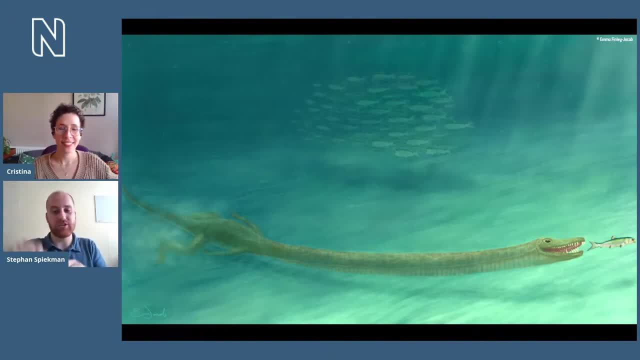 crocodiles and birds belong to, so the very, very base of that lineage this animal lived. and yeah, so the reason this animal has puzzled humans or scientists for so long is that it has very, um weird shape that is unlike anything that's alive today. right, so, sometimes. so that makes it. 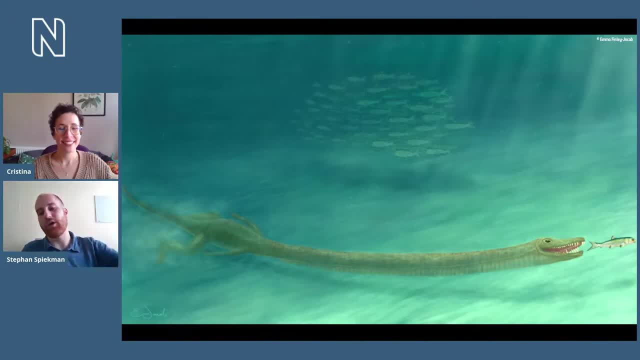 very hard to say how this animal might have lived and if this very long neck that might indicate it was living in water. we also even have some stomach content that indicate that this animal was eating fish, because we found fish skills in its, in its, in stomach content and at the same time you have 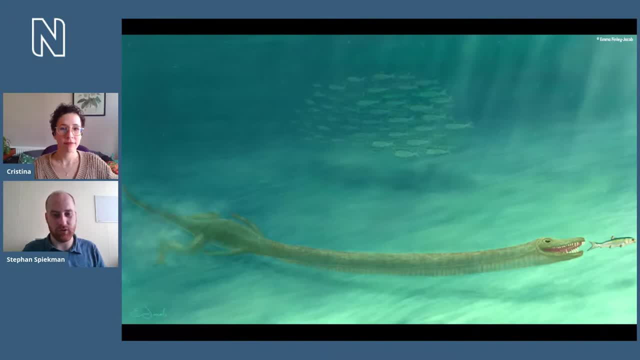 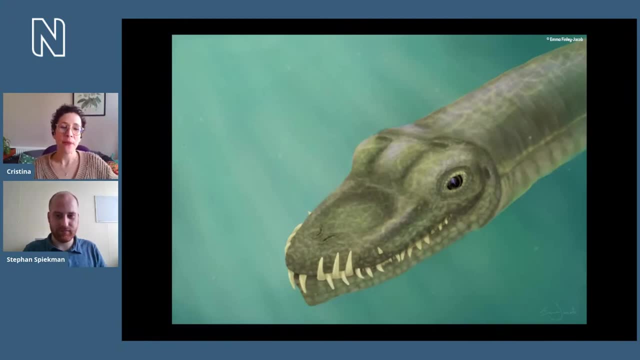 limbs and no clear adaptations for swimming. so there are no paddles or or fins, so it makes it a very weird animal, absolutely so. uh, stefan, where? where is tannister first? and tannister stanis trophy. sorry about that, i found, and can you tell us a little bit more about that area? 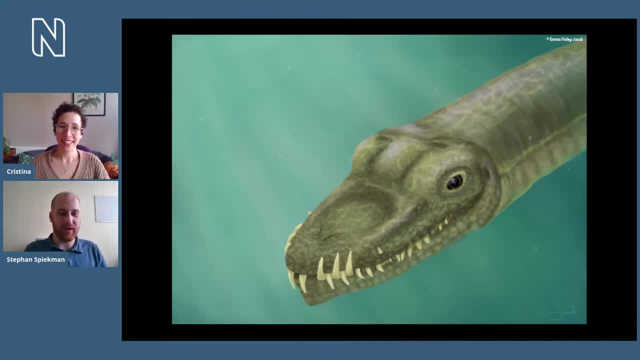 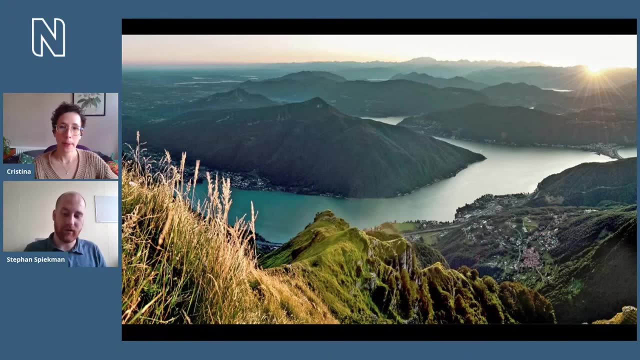 yeah, so tennistrophius is um known from a number of places in europe and also in china. many fossils have recently been found, so we do find this animal spread, but most of the best fossils, almost all of the best fossils, come from a single locality. 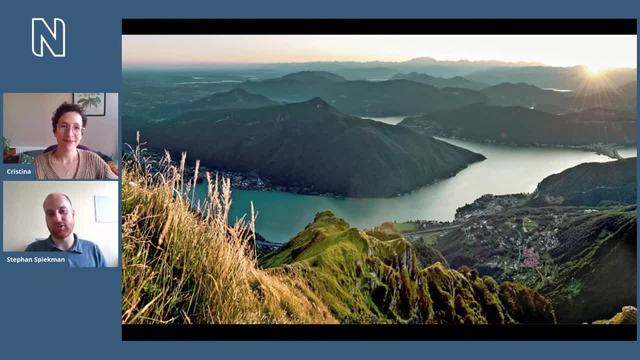 which is a real, actual dragon mountain. it's called montesan giorgio, it is located on the border between switzerland and italy and it is an actual dragon mountain because it is a site where you find many of these fantastic marine reptiles that we're talking about today, so not only tennistrophius. 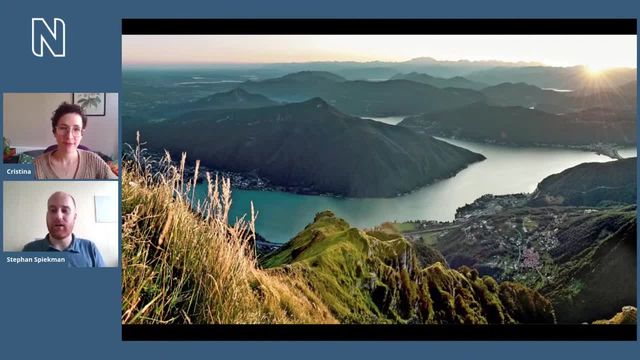 but also the placodons. we've been talking about the ichthyosaurs, um those ancestors of the the isosaurus. we all find them in this one mountain, and this mountain is so unique for its fossil fauna that it's actually been declared the unesco world heritage site because of it. that's amazing. 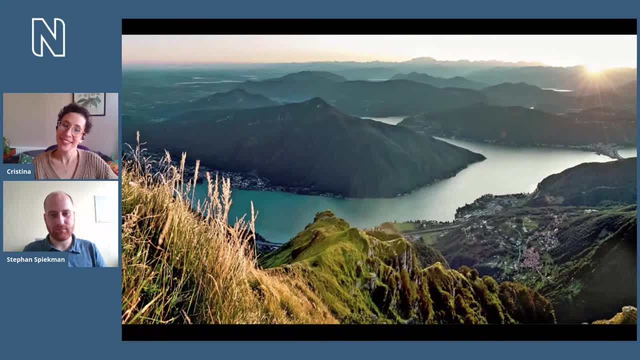 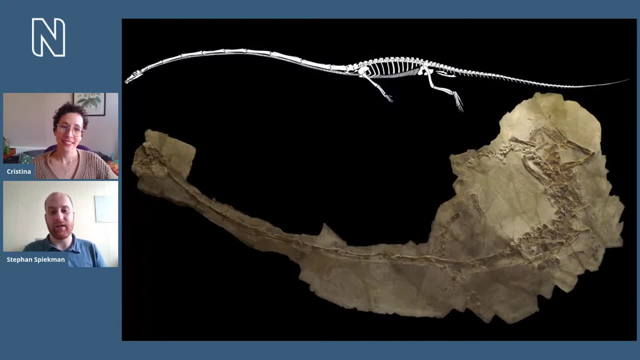 and how long have we known um about tennis trophies? so tennis trophy is the first remains of tennis trophies were actually described already in the in the 1850s, so you know over 170 years ago now and, as you can see here, you can get a better idea of how weird the anatomy of this animal. 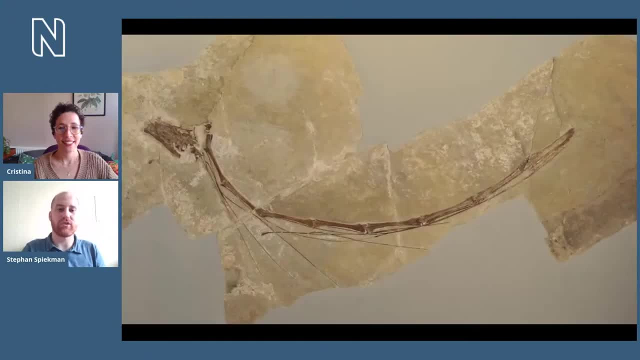 is. so you can see that this neck that is so long is actually composed of vertebrae that are extremely, extremely elongated. so the neck bones are extremely long and these are actually the first things that people found, that the research has found. so back in 1850 they just 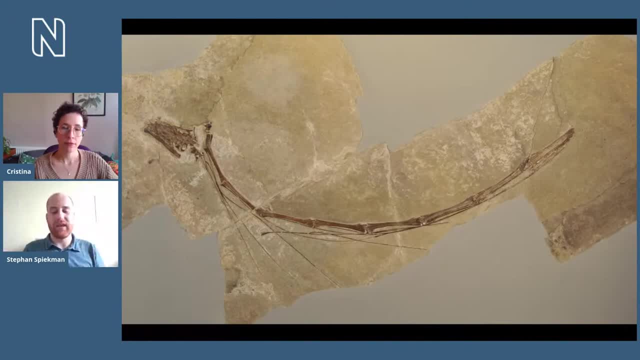 found individual bones that are about you know this long, and they were like: well, what are these things? we have no idea. some thought that there might be leg bones. uh, they're not. that they might have been interpreted as the the tail vertebrae of a certain dinosaur, but only later on, when we 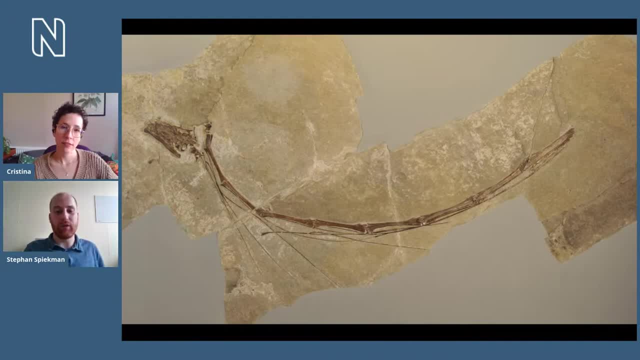 found these more complete skeletons that we're looking at now, uh, that we realized that actually. well, they belong to the neck and these and these fossils. they were only discovered at montesant, giorgio, basically from the 1920s onwards. that's amazing. and since since then, since the beginning? 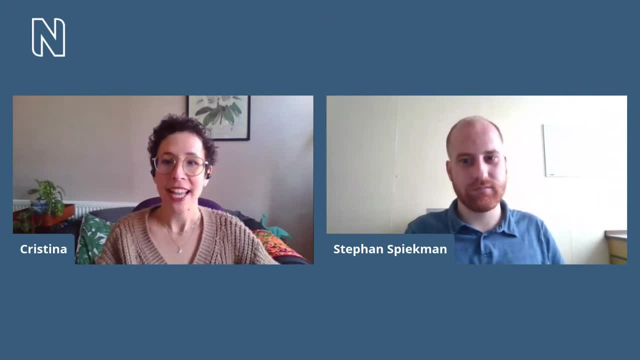 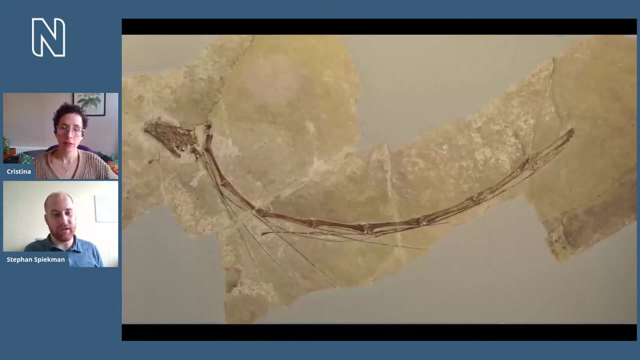 it looks like it's been puzzling scientists, as we said before. and why? why was the neck so confusing? because of this big vertebra that you were. you were saying is: definitely yeah, yeah. so essentially this, this neck is um built unlike anything else in the animal kingdom, so we have these vertebrae. 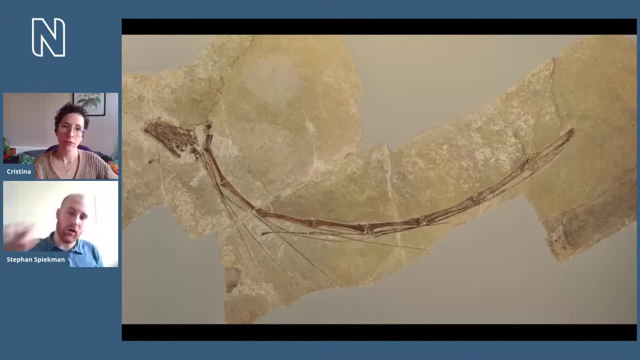 that are extremely, extremely long. and then underneath you see these long, strut-like things. so these are actually ribs. so reptiles, most reptiles- there's another reptile character for you: reptiles have ribs also in their neck vertebrae. so not only as we do on our, in our chest, in our torso. 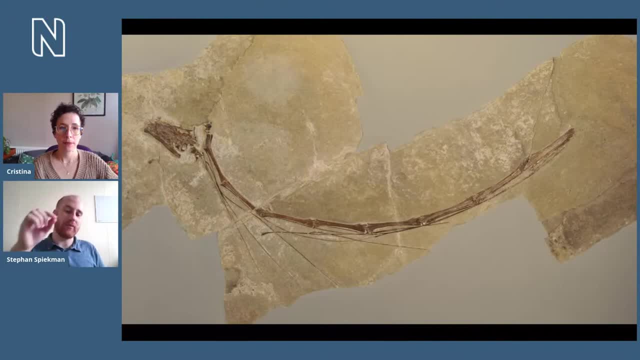 but also in their neck, And in telestrophius, these neck vertebrae became so extremely long that they covered the length of up to three or four of these vertebrae, So they would have overlapped each other and forming a tight bundle, keeping this neck supported. 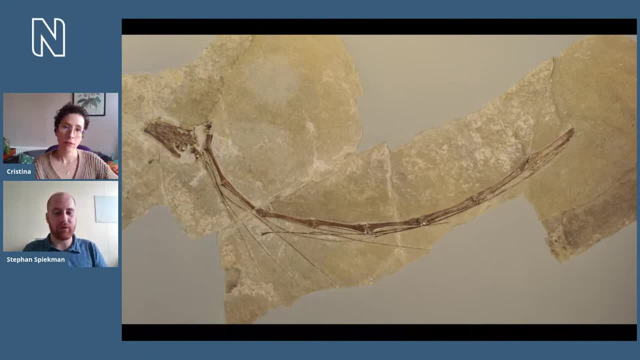 So basically allowing this neck to be stable, but probably also stiffening this neck. So it's a very weird construction, a very weird configuration, And we think this neck was actually quite stiff, so not very movable, Which actually links quite nicely with the different theories about how he lived. 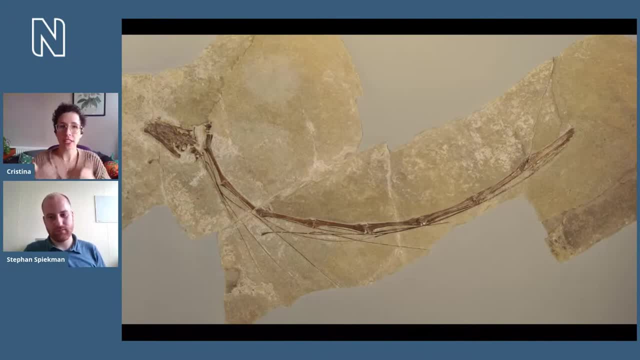 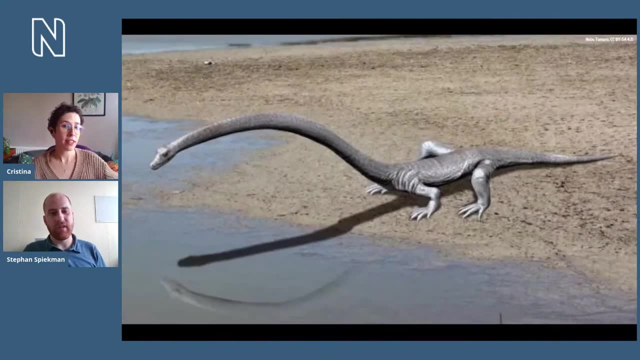 and how he ate, Because the old fashioned representation of telestrophius was that he lived on land, right? Yeah, so there've been many, many hypotheses through the ages, basically because everybody has a different opinion on this animal. But one of the more common ones and long standing ones, 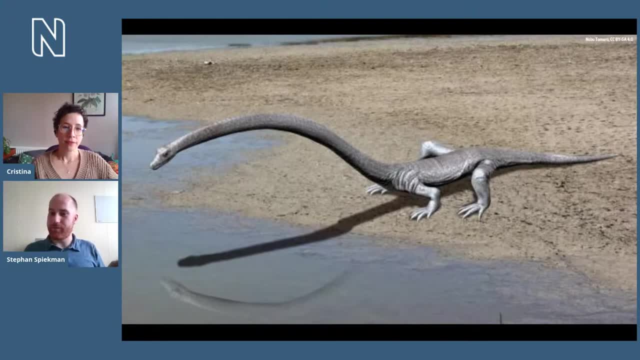 is that? yes, we know that telestrophius ate fish, but with his long neck maybe it was sitting on the edge of the water, on the shoreline, and using its neck, maybe like a heron, to snatch its prey from the water. 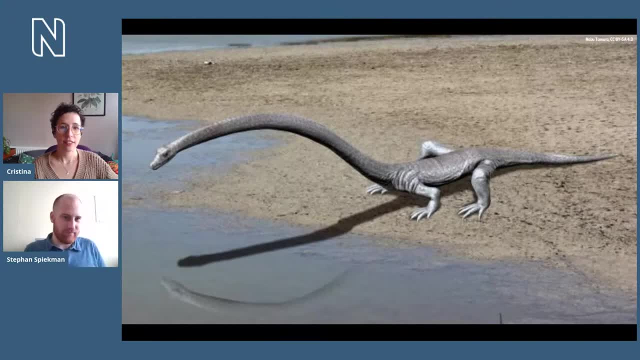 Then, when we later discovered that this neck of telestrophius is so stiff, this became a more unlikely hypothesis. But there's still some people today who think that telestrophius might have lived like this. Now, Stefan, we're talking about telestrophius. 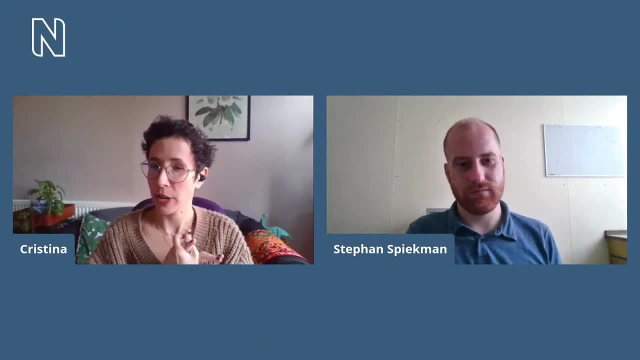 as one animal, but there are two kinds of telestrophius Right, And actually I think that's a good question. Actually, Erica, from our viewers they were asking how big were these creatures? And I think the answer is coming up in the next question. 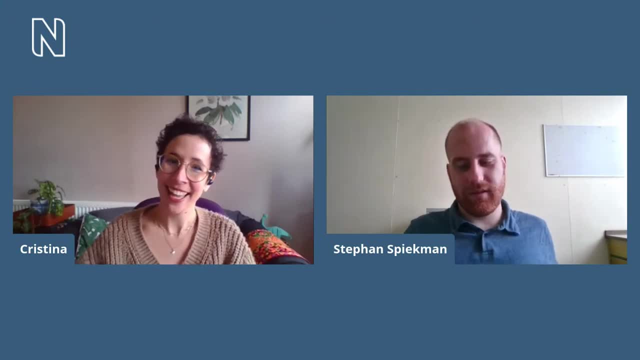 because tell us about the two kinds of telestrophius that were out there. Yeah, so, as I said, most of the telestrophius fossil all come from this one single mountain, the Monte San Giorgio, And on this mountain we find two different types. 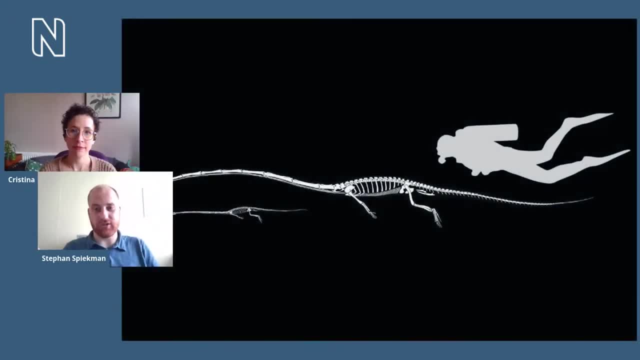 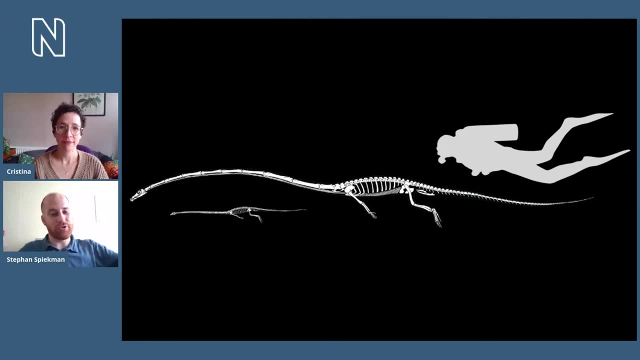 of fossils of telestrophius, We find pretty big ones, which are the skeletons we've been looking at so far, and they could be up to five meters long in total, So a very long animal, which shouldn't give you the impression. 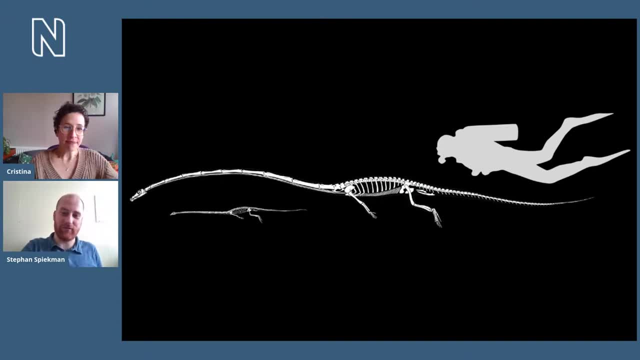 that this was like a big, ferocious animal, because if you look, for instance, at the torso of this animal and put it next to the torso of a human, you see that the torso is more or less similar. It's just five meters long because this neck 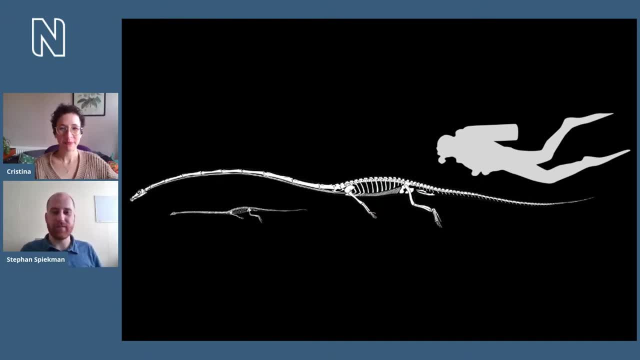 is so incredibly long and the tail, similarly, is also very long. So that's the large form that has been found in Monte San Giorgio was about five meters long, And then the other form we find are all fossils that are a lot smaller. 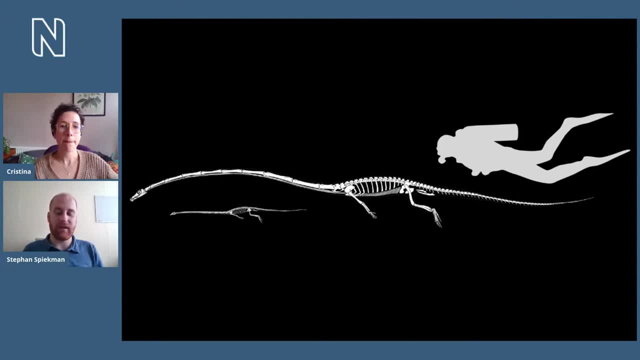 They're about like a meter to a meter and a half In total length And, yeah, they were both found at the same mountain And historically they've been considered, for logical reasons, as the juveniles and the adults of the same species, so as the babies and the grownups. 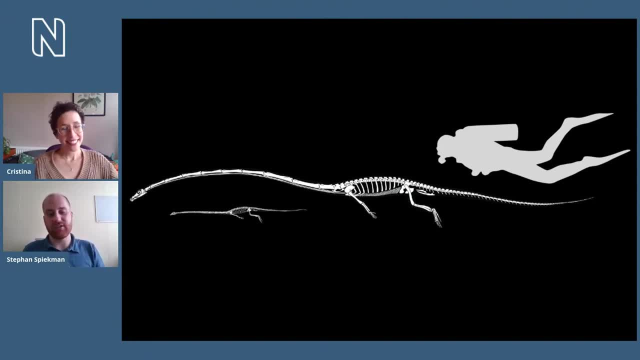 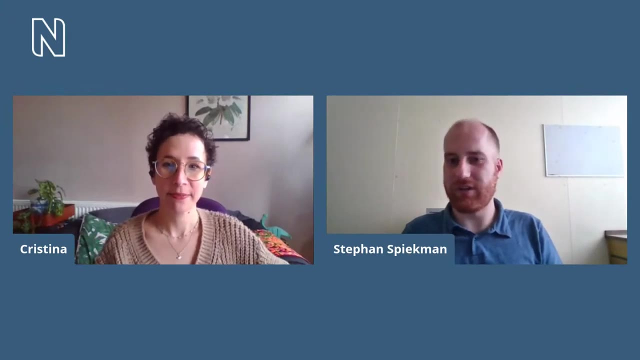 But there are some differences between these two forms other than their size. So there was already an indication that the skull of the large form and the small form are actually quite different, And this is something that I wanted to investigate in my PhD research to try and figure out well. 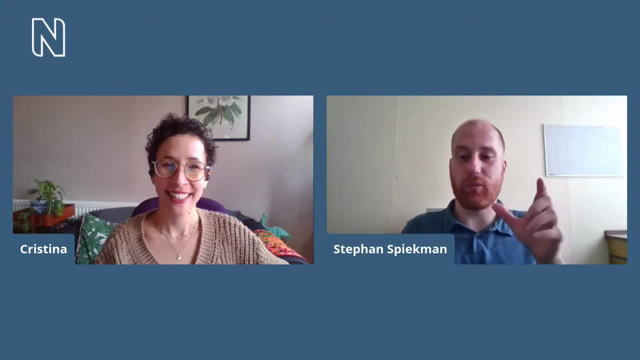 is this actually going on or not? Because the weird thing is that the small form has different teeth compared to the large form. So the small form has tricuspid teeth that might be used for crushing things a bit more, whereas the large form has very long and piercing teeth. 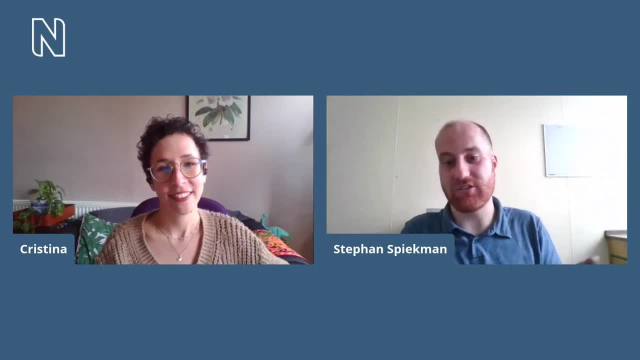 And so people have suggested: well, maybe the babies were just eating something else than the adults. But actually it would be quite a unique transformation for a reptile to make this three-dimensional. So we don't see this in many other reptiles. 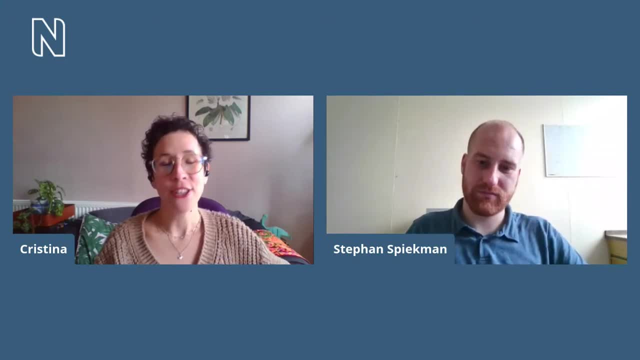 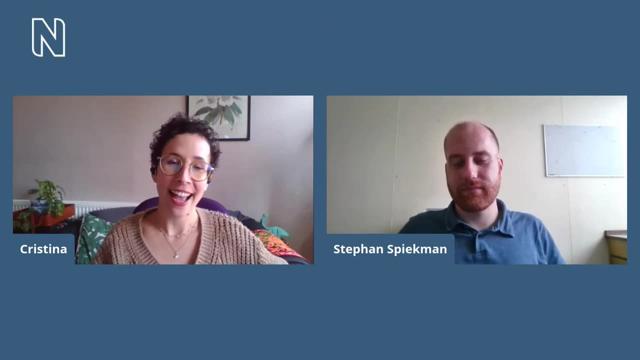 We don't see this in many other reptiles, And you did. you have studied them, Stefan, and actually you've come up with to our conclusion. Have you figured out whether they are different species or juveniles and adults? Can you tell us? 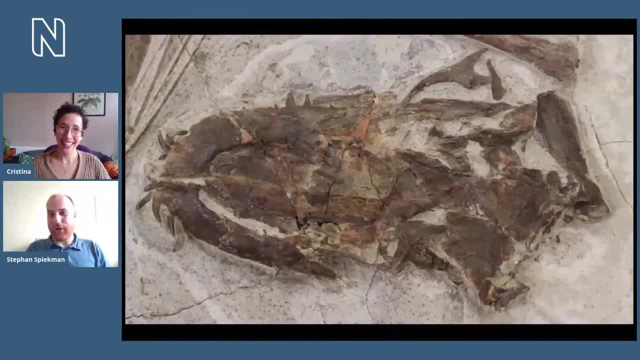 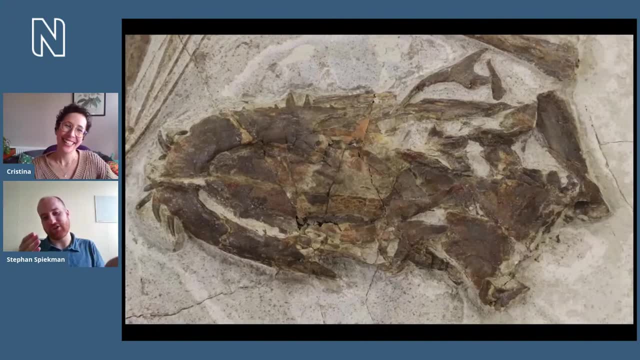 Yes, so what we did is, so I'll keep the answer. Well, I guess people can guess the answer, but I'll come to that in a bit. But basically, what we did is in trying to compare the small form and the large form. 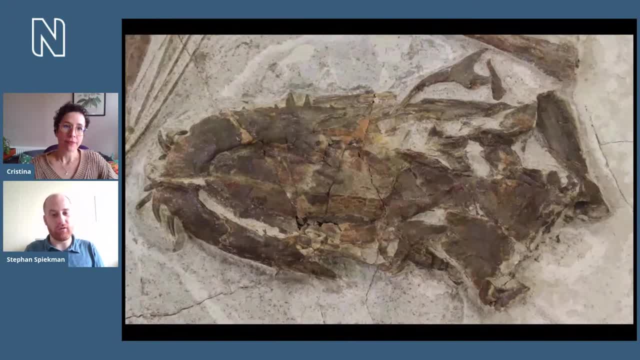 the problem was that we didn't know really how well how the skull of the large form looked like. This is because we have a number of fossils of them, as the one you see here, but they're all very strongly crushed. So after fossilization or during fossilization. 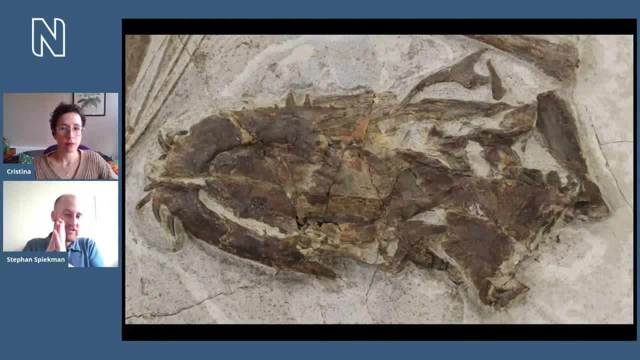 there were many geological processes going on which made that these skulls were all very compacted and crushed together, which obviously makes it difficult to understand how this animal might have looked like in life. So we had a better idea of how the small form looked like. 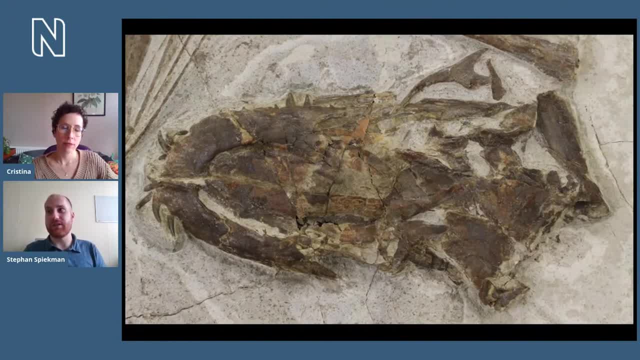 but not as good of an idea of how the large form looked like. But nowadays, in let's say the last 15 to 20 years, we as paleontologists have a new, very strong tool that we can use to investigate these animals. 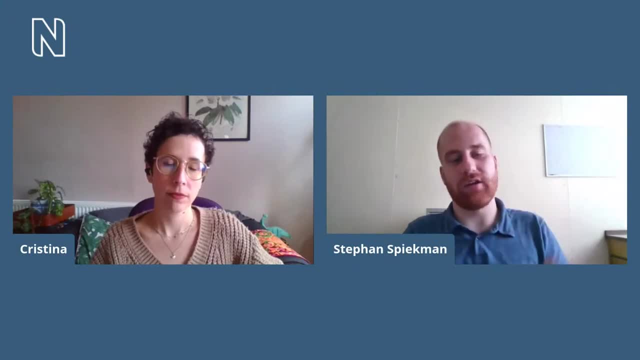 which is CT scanning. So we scan a lot of fossils to give us an idea of how these animals might have looked like, to look at fossils that are difficult to study with the naked eye, And this is what we did with this skull that I just showed you. 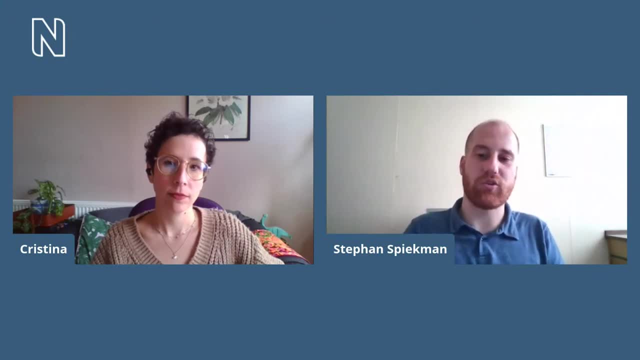 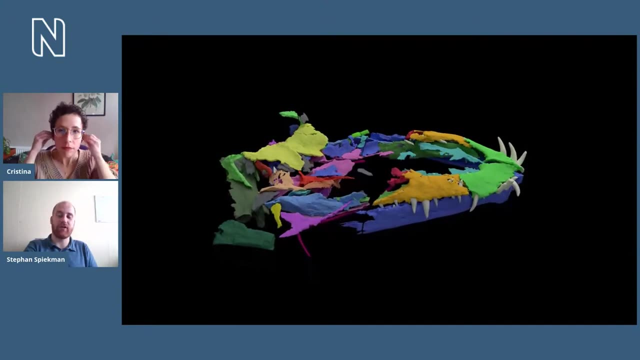 We put it in a very strong CT scanner and then I spent a lot of time trying to segment well, to digitally prepare out all the bones essentially, And we ended up with this final model And, as you can see, there are many more bones. 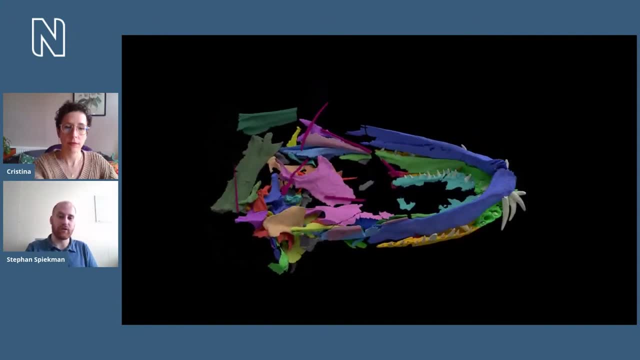 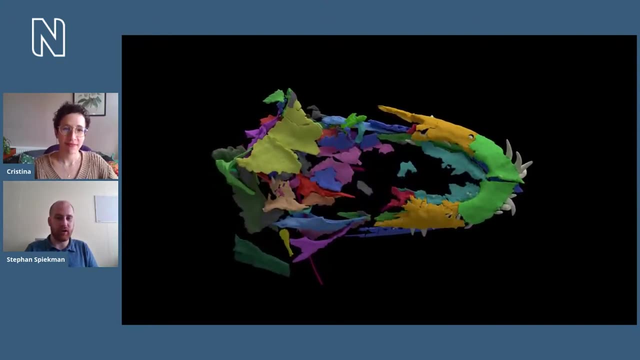 that are visible than are with the naked eye, especially here. now that we look at the bottom, There are a lot more fossils that were preserved in the stone that we couldn't see before. It gave us a lot more insight in how the skull might have looked like. 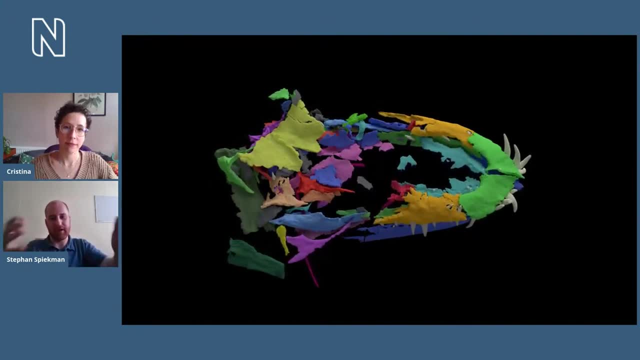 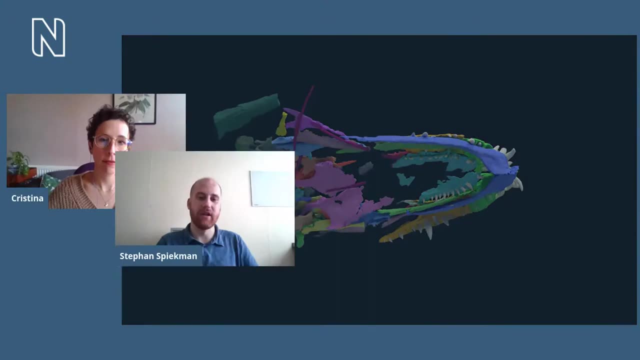 But you still don't really have an idea of how this animal looked like in the flesh, just because, well, it's all still. all the bones are displaced, It's all crushed together. It's a bit hard to see. So what we then did with these digital bones? 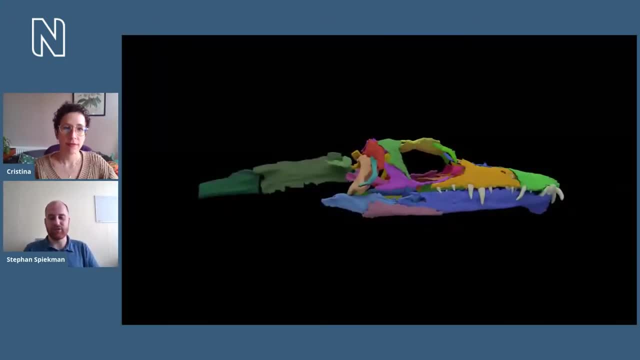 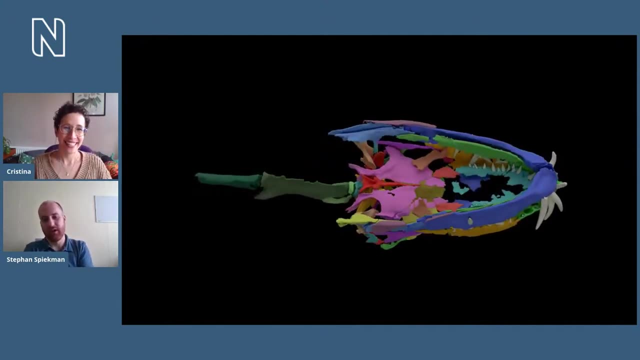 is basically puzzle them back together in the position they would have been in life, which eventually resulted into this really nice reconstruction of the same skull. This is all from the one fossil we just showed you And, yeah, as you can see, most of the skull is there. 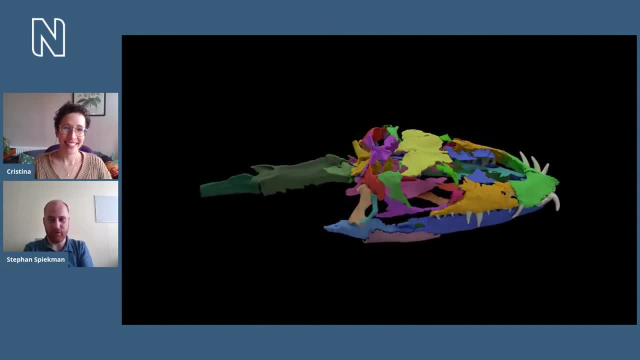 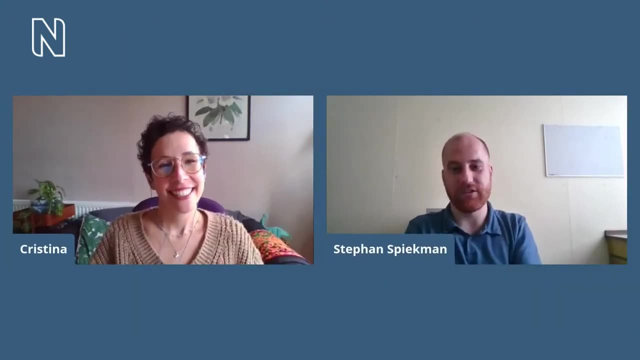 There are a few pieces that are missing, but really virtually complete skull was hidden in that rock. So that was really exciting, obviously, when we were able to finalize this model And it allowed us to compare this large form in a lot more detail. 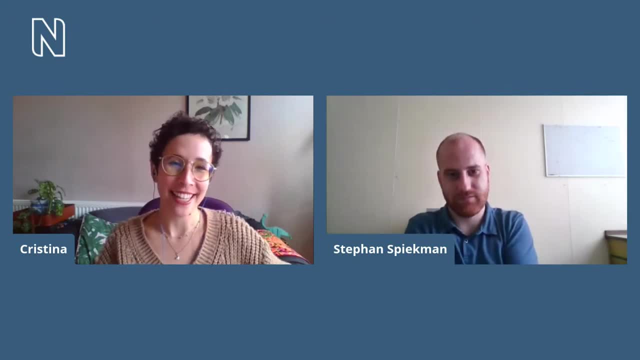 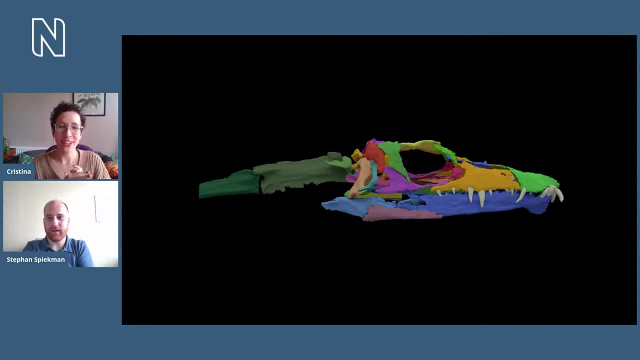 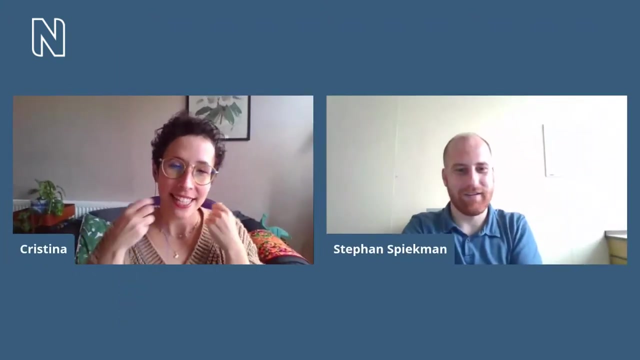 to the small form. I'm sorry I can't hear you at the moment, Christina, I think you're muted. Yeah, I think that's fine, So that I was gonna say that that's the beauty of science and seeing the image crushed, and then 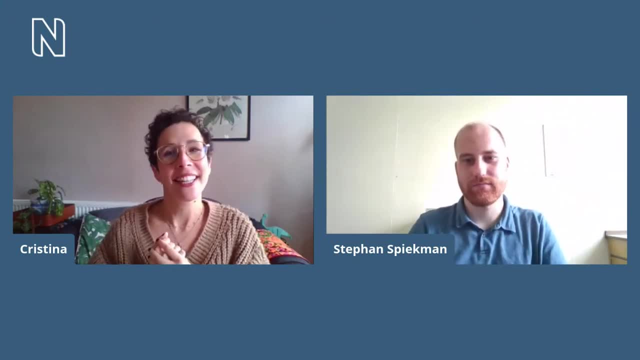 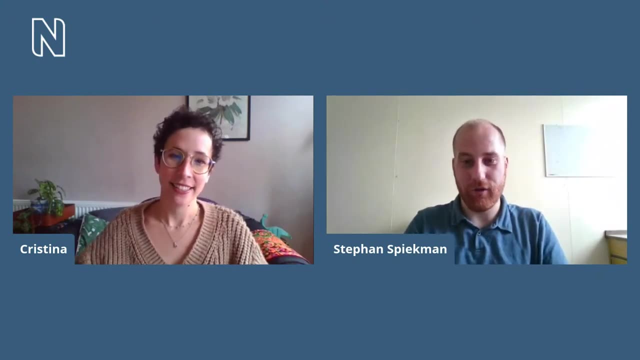 and then in 3D over there. But can you give us the answer, Stefan? Is it young and adult, or two different species? So yeah, I think we have. on the following slide we have the skulls next to each other. 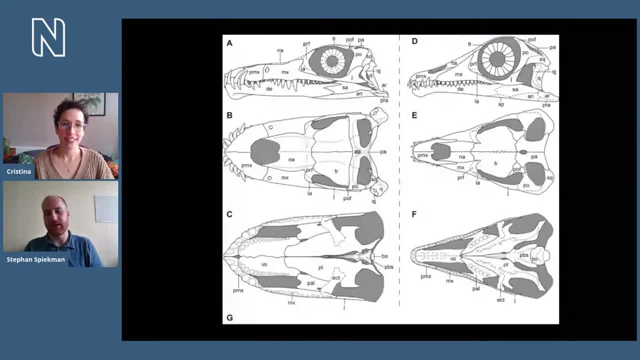 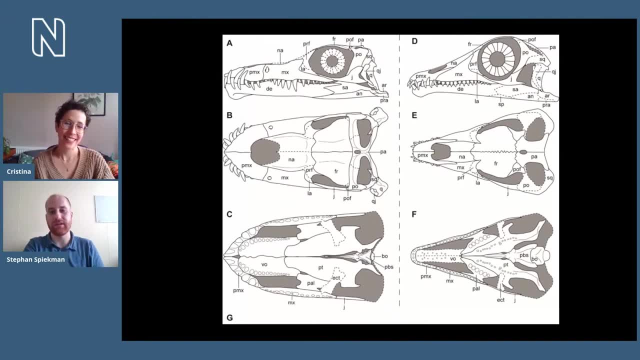 So you see how the large form looks like and the small form looks like, and then you can see that there's really a big difference. So on the left we have the large form and on the right we have the small form, And you see the difference in the teeth. 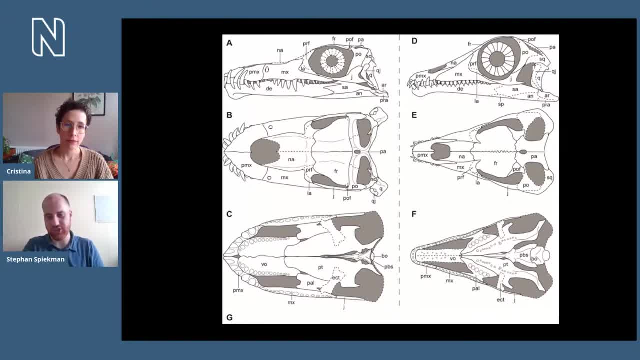 that I was talking about earlier. but you also see that just the general shape of the skull is very different. And in the two bottom pictures you see actually the roof of the mouth, So the what we call the palate, and you see, that's also very, very different. 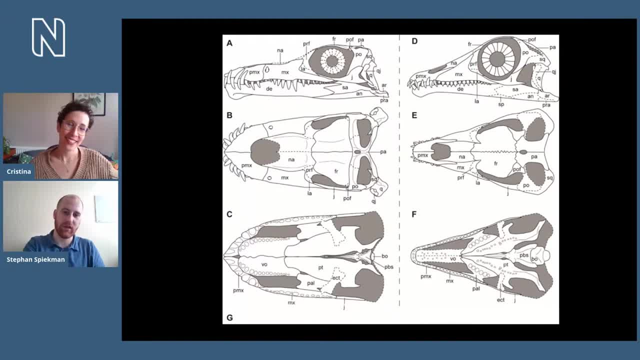 between the two forms. So you see that the large form only has a few teeth in the roof of the mouth in the front, whereas the small form had basically teeth all over the roof of the mouth. So these are really two different species. So we were quite convinced after seeing this. 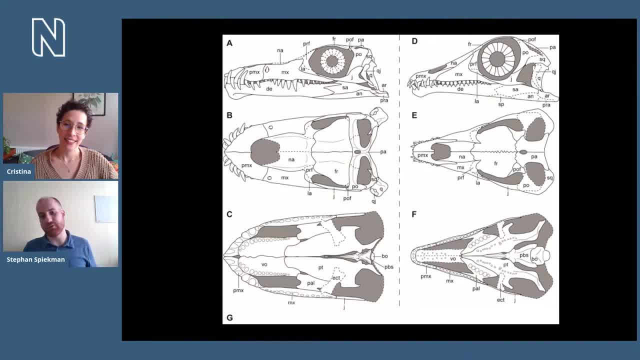 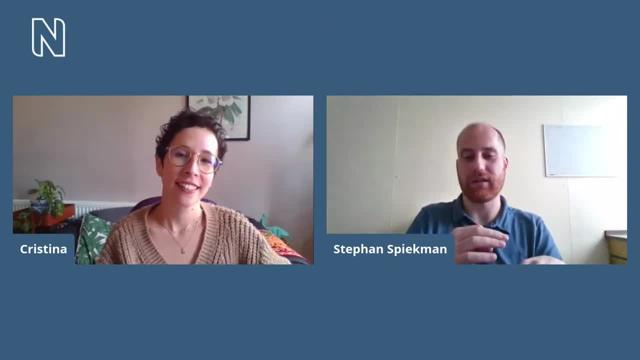 that they were two different species. But in order to be really, really sure, we did some additional research where we basically took one of the bones of the small species and took like a thin section and looked at it under the microscope and looked at the growth lines. 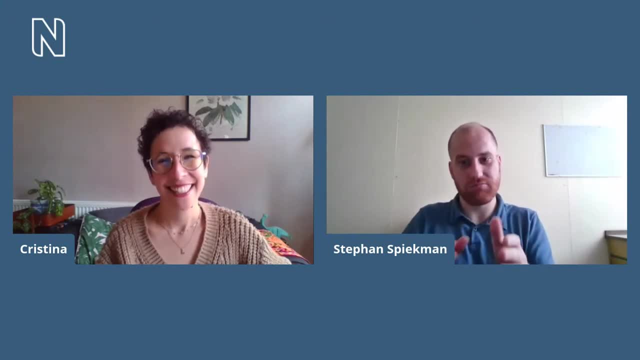 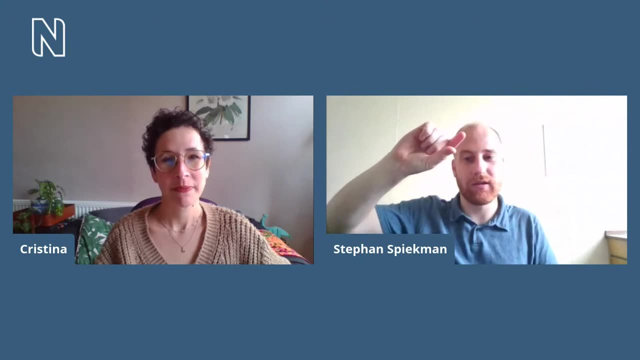 And based on these growth lines, we could see that actually this small form was quite old actually And we could even see in the type of the growth lines that they were very closely bound together at the outside of the bone, that towards the end of the life of this animal. 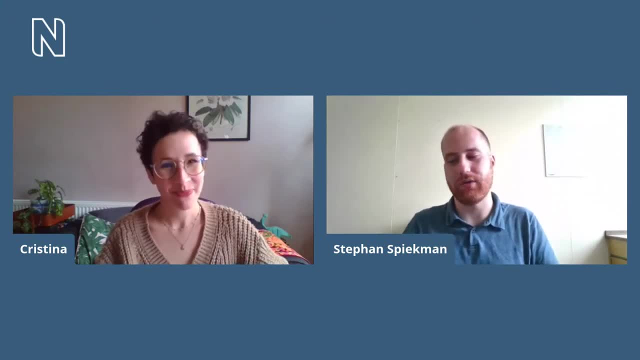 it had basically stopped growing because it had reached adult size. So we really have now very, very strong proof that these two species, that these were two different species, And that's of course very interesting, because then you have two different species of tenostrophias.